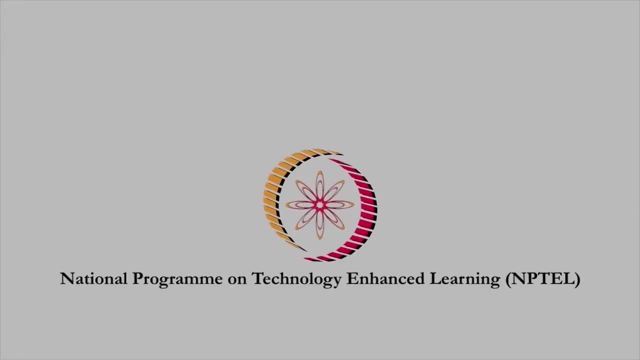 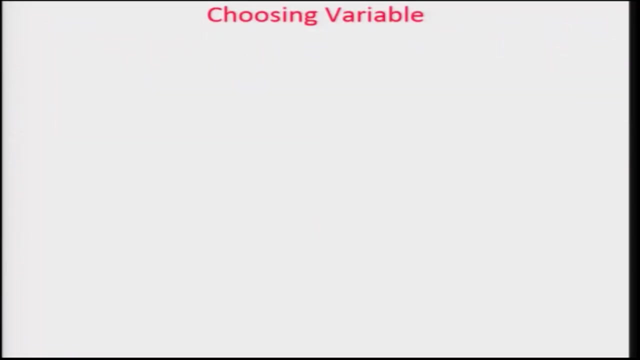 So, continuing on to the simple example, as we said, we were trying to find out how a student will travel from cheapest possible from Kanpur and visit 3 college cities. Now let us start focusing on the first aspect of it: choosing variable. So the most important step in building. 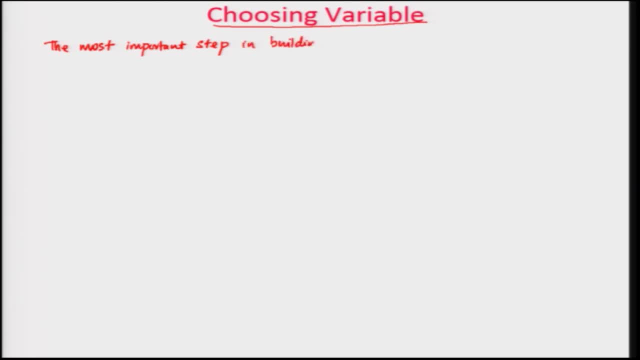 a model is to decide on, Decide variables that will facilitate modeling. So the most important step when you want to build a model, the most important step is to decide the variable that will facilitate modeling. In many cases when you try to build model, as I remember, 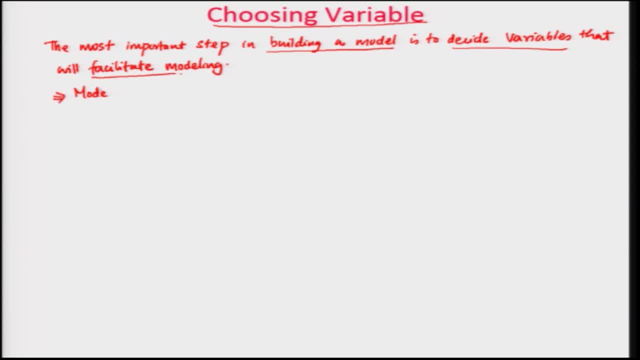 Modeling is usually done by hand. Modeling is an individual exercise done by hand or done by an expert. Individual does the modeling, So the choice of the variable is typically left to that individual. And this choice of the variable, or the decision on which variable, 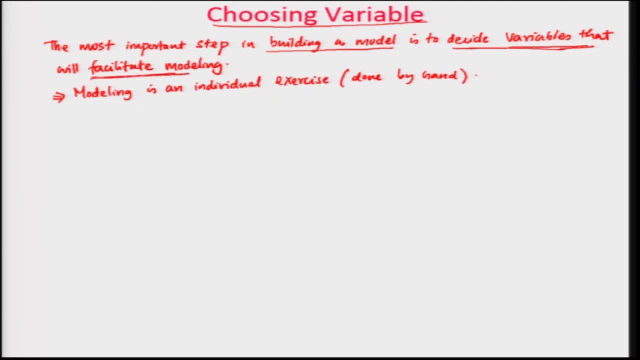 to use influences, the. it facilitates the modeling process. okay In this example. okay, any round trip. any round trip consists of a series of series of smaller trips. okay, between two cities. so any round trip in our model consist of a series of small trips between two cities. what we do is: it makes sense. it makes sense to assign variables. 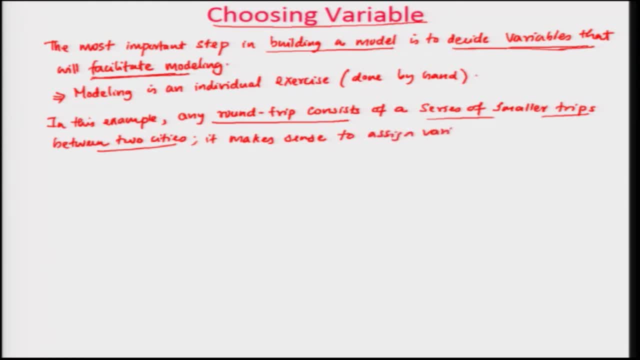 okay, To assign variables to the decision, to the decision of whether to travel, whether to travel from one city to another city, okay, Okay. So here, what you are trying to do is you are trying to make the decision. your decision is once you reach Bombay. okay, so the idea is that, from Kanpur, where do you want to go? 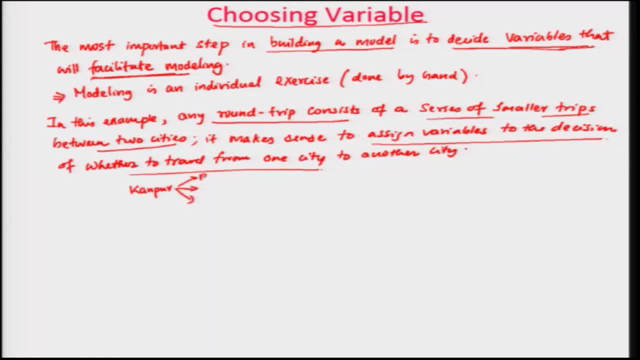 you have three options in front of you. you can go to Bombay, Delhi or Madras. okay, From here. once you decide I want to go to Delhi, let us say, for example, or you want to say I want to go to Madras, then you have only two options in front of you. that is either. 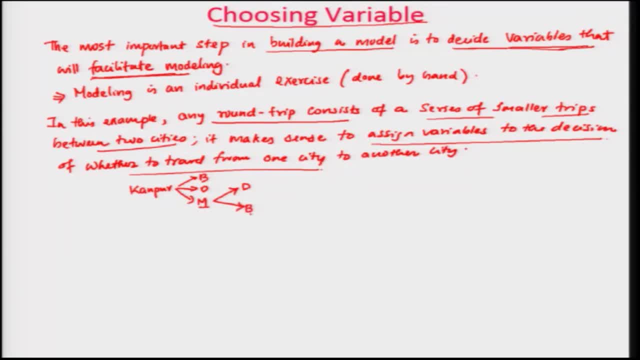 you can go to Delhi or go to Bombay. okay, Okay, Okay, Okay, Okay. I want to go to from Madras, I want to go to Bombay. then there is only one option in front of you: to go to Delhi, and from Delhi then you have go back to Kanpur. in that regard, 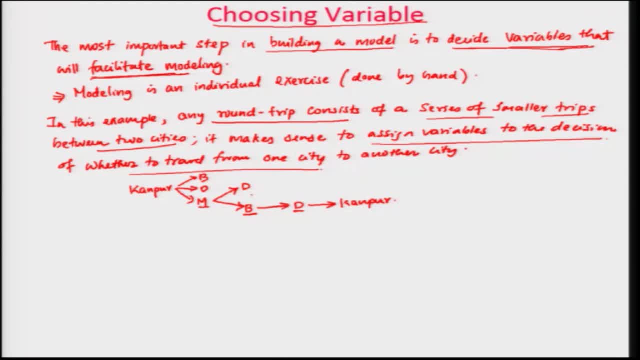 okay, So depending upon which you choose- your path or your- the order in which you visit the cities will change. So what we are trying to do is whether to travel from one city to another city. whether you want to do that option is what we are actually trying to model. that is what the 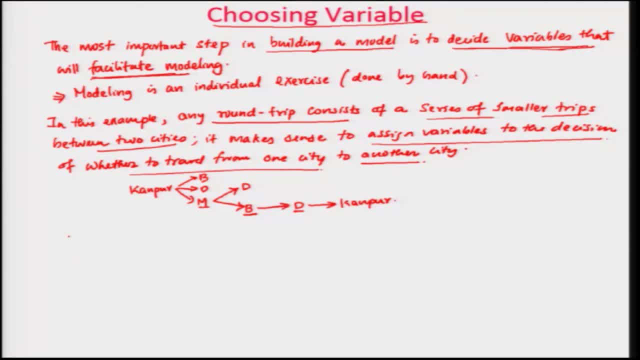 variable that we are trying to do, okay, Okay. So if there is a variable, if there is a variable, X12, okay, which implies okay, which implies student traveling to city, Okay, Okay, City 1, you realized from city1, okay, and in this case city1 is Kanpur. 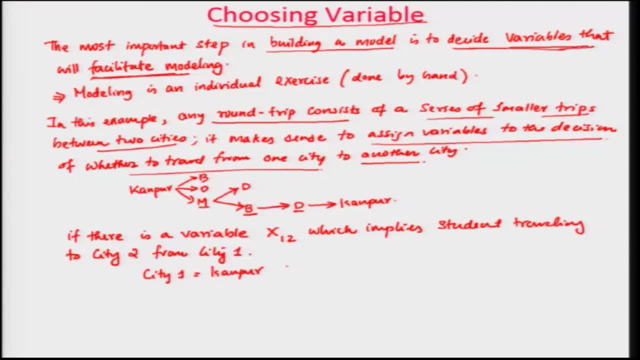 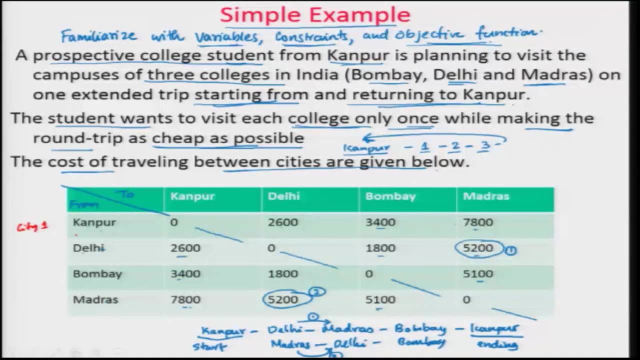 City 2 is city two, in our case will be Delhi. How did I get this? The answer to that question is this: is our city1? okay, Kanpur, Then. or you can think about why, then? or you can think about it as a city 1, okay, city 2, city 3 and city 4: okay, same. 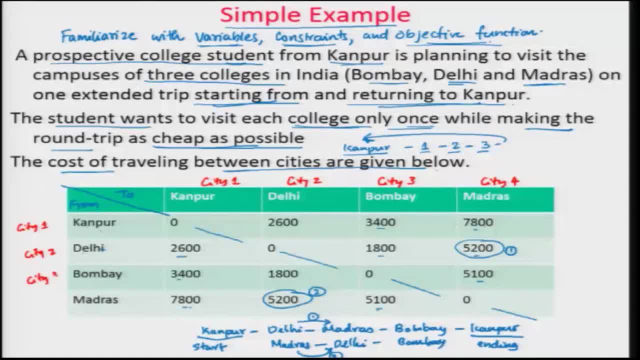 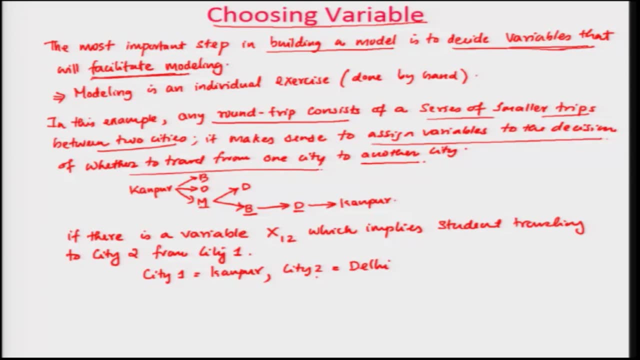 way: city 2,, city 3,, city 4. okay, So this is the. so in this case, I can think about these as the cost of the travel okay, and X12 is pretty much a travel okay, whether this student will travel from city 1 to 2. 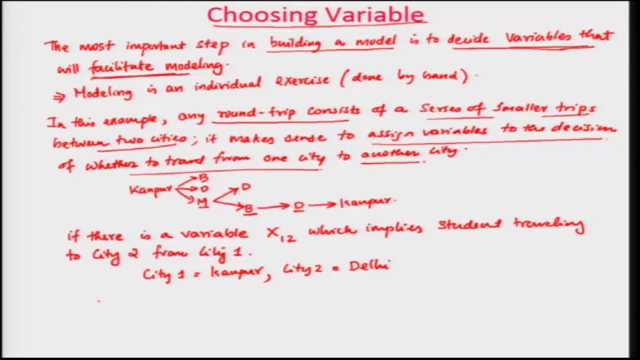 in this regard. okay, So if student travels, then X12 is equal to 1, which means the student will travel from city 1 to city 2.. If student does not travel, Then X12 is equal to 0. okay, So what we are saying here is that the student does not travel from city 1 to 2, it actually 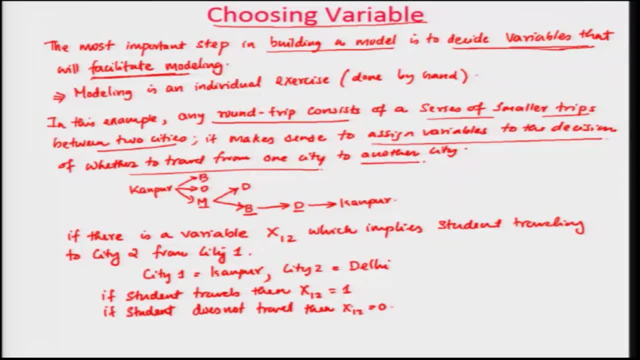 went to some other city. So the value of this travel is that the student will. this basically says: that tells you whether the student can travel from city 1 to city 2.. Then there is nothing important about city 2.. Then there is nothing important about city 2.. 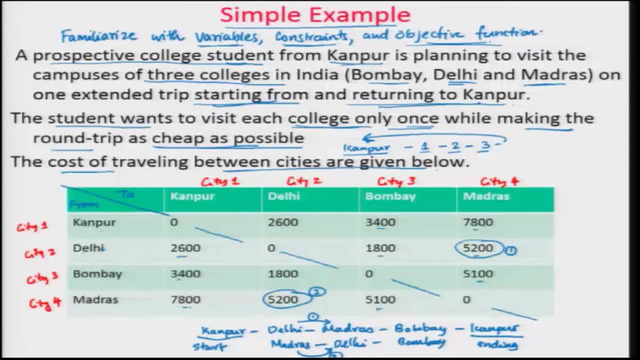 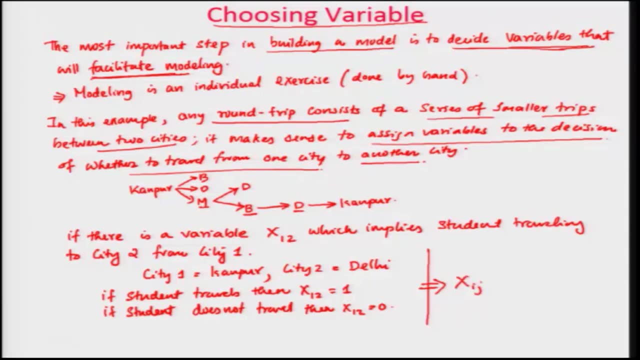 If you think about this and I am going to, let us say, use these indexing, go through this as with index- as j and I am going to use this as index of i, So then I can make this variable as Xij, okay. Xij means the value of i can vary between 1, 2, 3 and 4. okay, and j can also vary between: 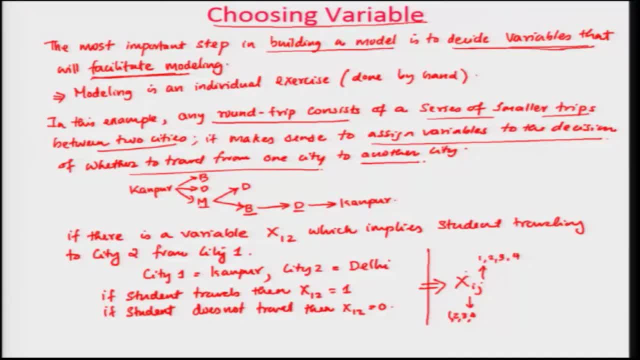 1,, 2,, 3 and 4. okay, So this will give me back the value of xij. So this is the value of xij. So this is the value of xij. So this will give me, by changing the indexes of i and j, I can model any travel from any. 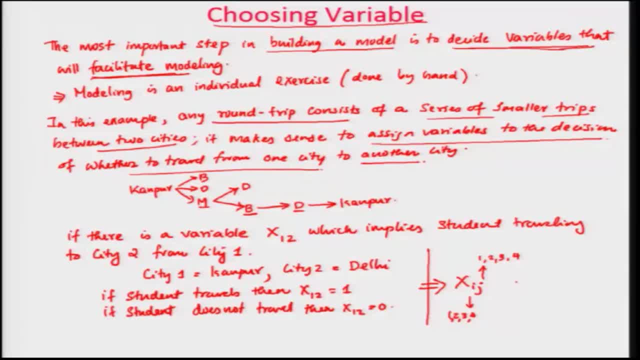 city to another, okay. But then there is also one thing you should notice that not that okay. there is no such thing. there is no such thing as trip to the city itself. So this is the thing. This is the thing. This is the thing. 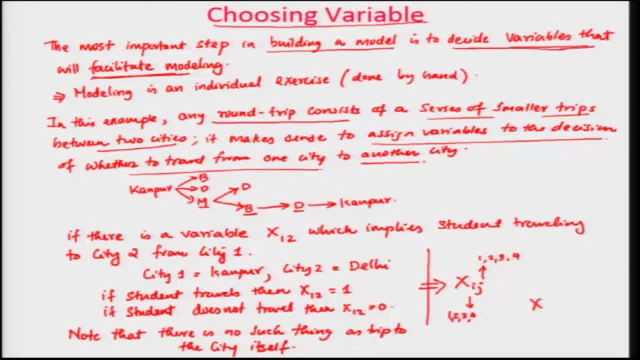 So when I am saying is that if I say X11, which means travel from Kanpur to Kanpur, This is always should be equal to 0. Same way, X22 should always be equal to 0.. X33 should always be equal to 0, okay, and same way, X44 should also always be equal to 0. 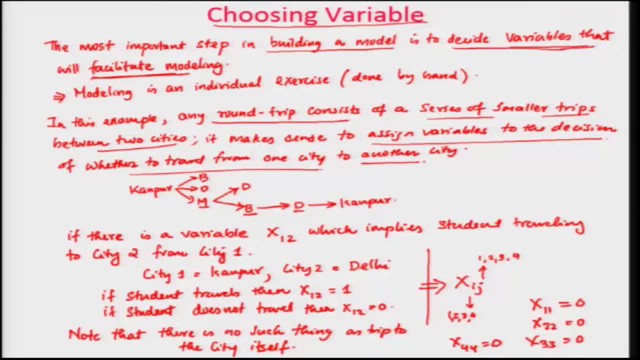 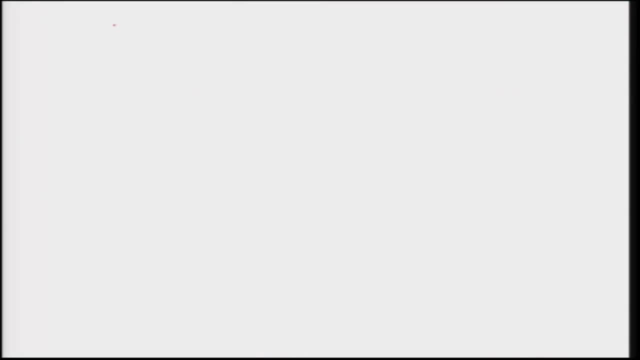 So if I have to say, for all these things, or if I have to write about this, Then the next major thing is this. So if I have to write about this, The next major thing that I have to do is I have to say xij is the variable, okay is. 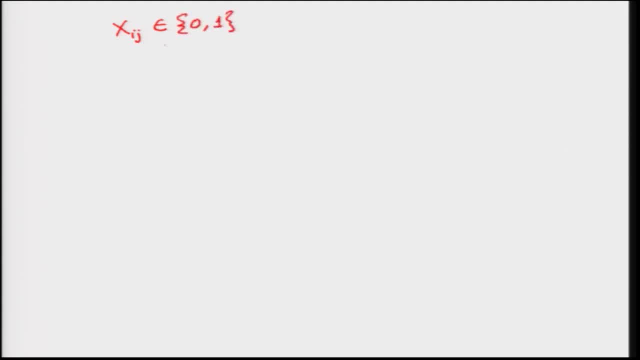 an element of the set 0 or 1.. Which means the variable xij can take any value. Okay, Okay, Either 0 or 1. okay, 0 means you are not visiting city i, So xij equal to 0 means do not. or the student not visiting not visiting city j from city. 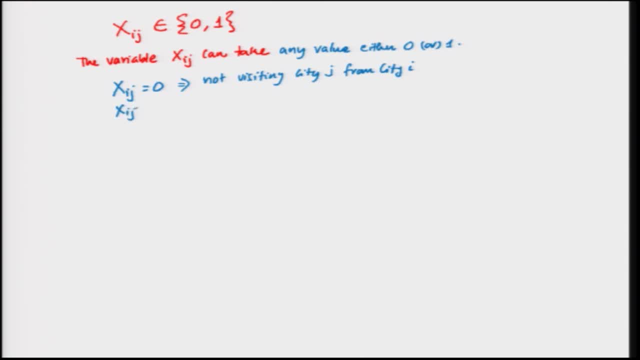 i. So if it is equal to 1, then you are visiting city j from city i. This is the yes and this is the no. All right, So if I have to write this down, Then if you can think about it as a proper way, is having a matrix. 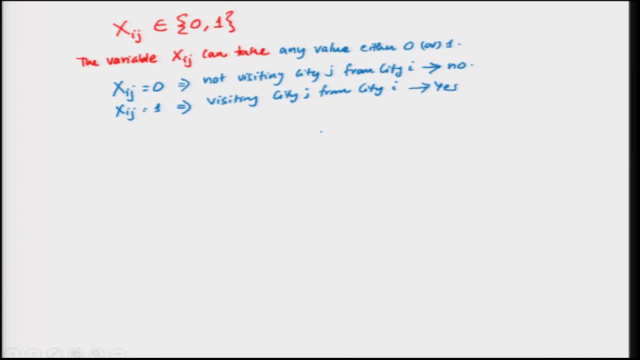 So the matrix is: There is no matrix. There is no matrix. Right, Got it Okay? okay, the previous matrix that we talked about, I can think about a scenario like this. okay, So we have Kanpur, Delhi, Bombay and Madras and same thing here: Kanpur, Delhi, Bombay. 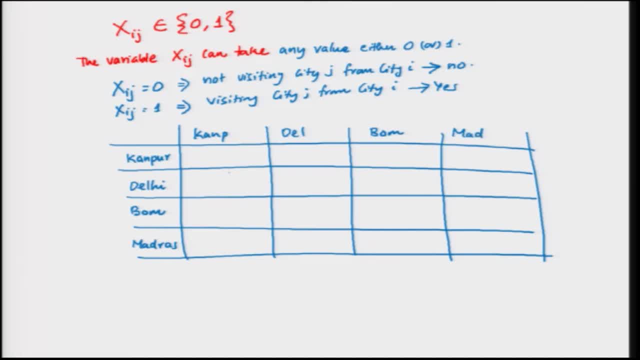 and Madras, okay. So if I and we said also that Xij equal to 0 for every i equal to j, Okay. Whenever i and j are the same, when they are 1 and the same, then these values are equal to 0. 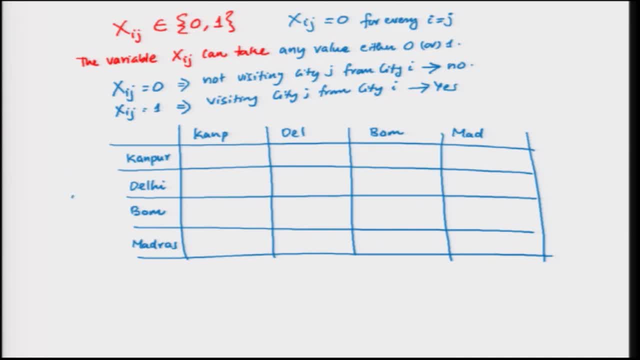 This is only possible when. so this is your index i and this is your index j. okay, So the variable is 1, 2, 3 and 4. this is 1, 2, 3 and 4.. So when i equal to j, this can happen is at this place. this is X11. this point is X11. 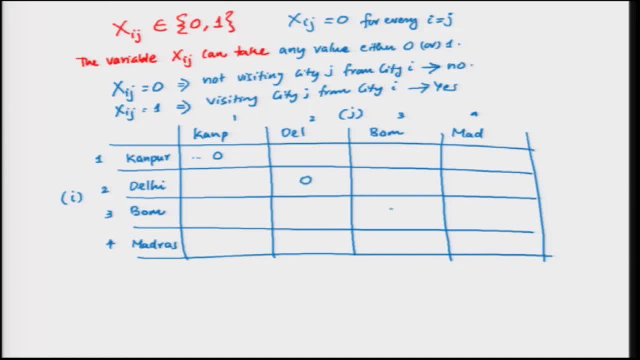 So this will be 0.. This is X22- 0.. This will be 0.. This will be 0 because this is Delhi to Delhi, Bombay to Bombay, Madras to Madras. So in all those cases where the index i and j have the same value, the variable will take. 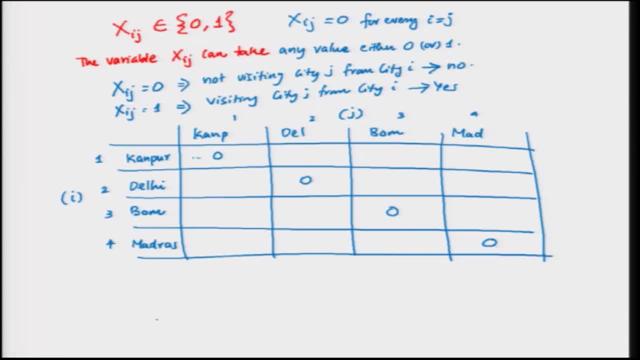 0, which means the tour within this city is not allowed. okay. And then if I write, if I do an example, if I do this like write this, okay, Then what does that mean? That means I am visiting from Kanpur, I am visiting to Delhi, okay. 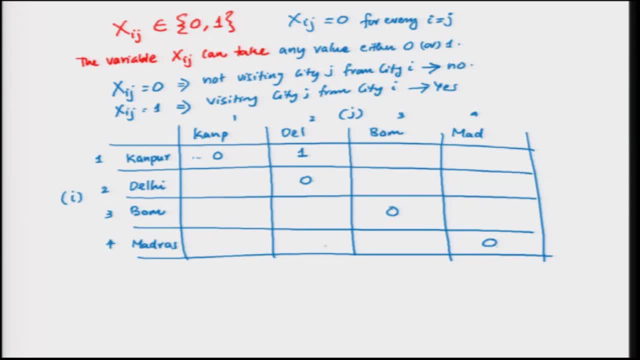 So, So that is the idea. okay, If I say something like this, then I am visiting Kanpur to Bombay. If I write something like this, then it is Kanpur to Madras. okay, If I do something like this, then it says I am visiting, I am coming back to Kanpur from. 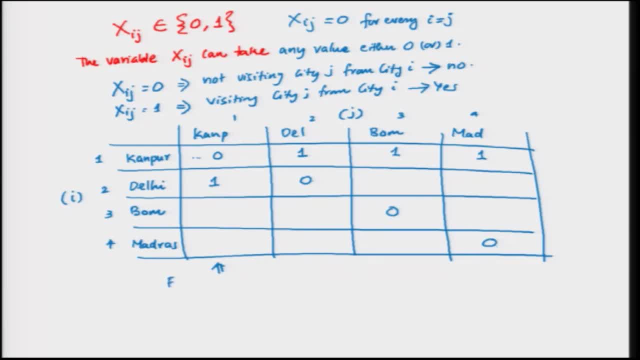 Delhi. So this column tells you from which city you are coming back to Kanpur. okay, Okay, So. So that is the idea in this case. all right, So the idea is, as I said earlier, so this Xij, this variable that we talked about, this is 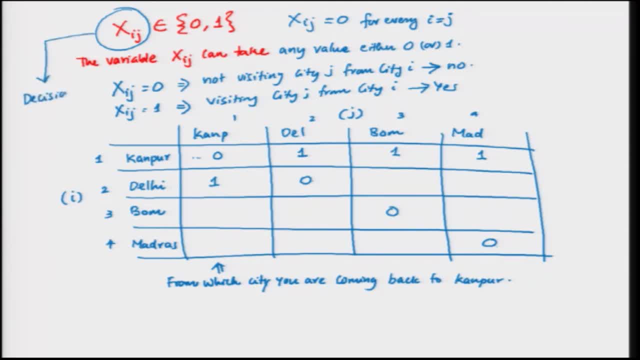 most of the time what we call as the decision variable. We need to decide, okay, whether to visit city j from city i, yes or no. that decision is. that is why it is called as a decision variable, okay, So So the decision is once the variable is chosen. once the variable is chosen, then the attempt. 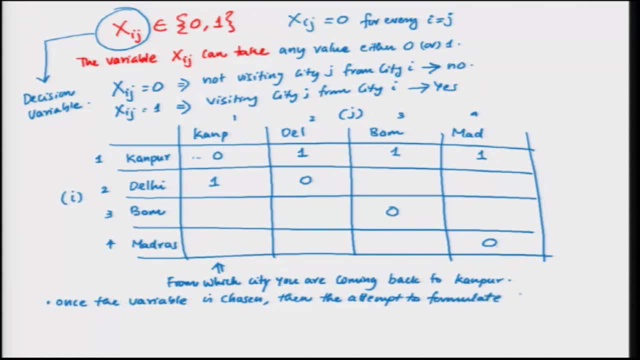 to formulate, attempt to formulate: the problem is made, problem is made. okay, So what you try to do, it is: You have chosen the variable. So then, once you have chosen the variable, then you try to attempt to formulate the problem. okay, If formulation, if formulation is difficult or cannot do it, okay, 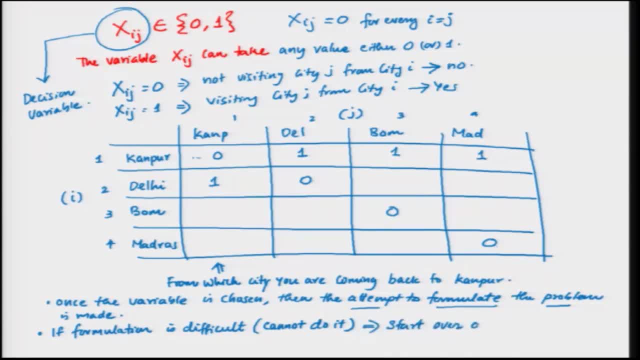 Then you have to do is start over, Okay, And define the variable, define the. define the variable differently. So if it is impossible with the current variable definition and you find it is extremely difficult for you to formulate the problem, then it is better to start over and define a new set. 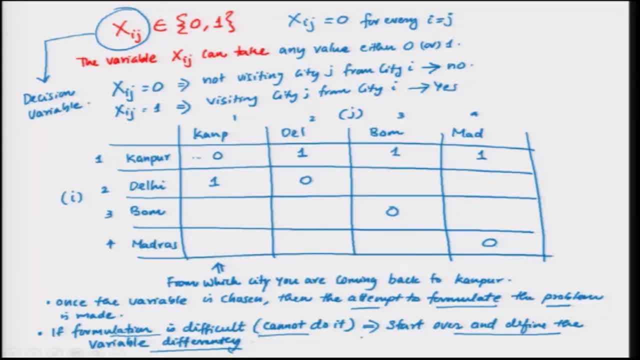 of variables, okay, And usually what happens is many a times okay. Okay, Variable choice is an iterative process, So one of the rules that you need to remember in this regard is this: Variable choice, or choices, can be an iterative process if the problem is complicated. 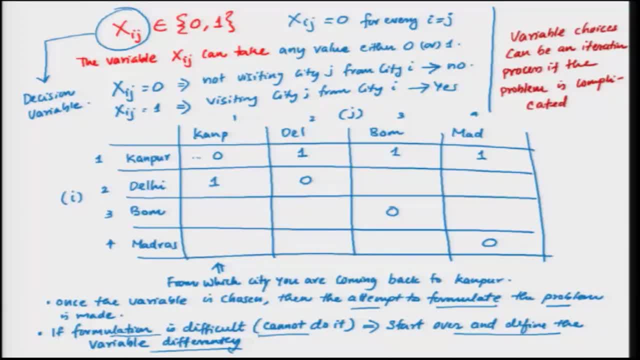 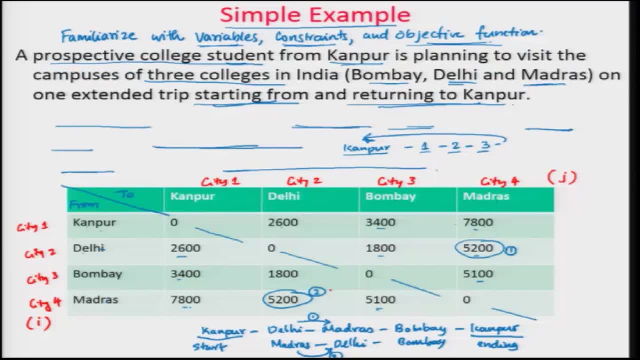 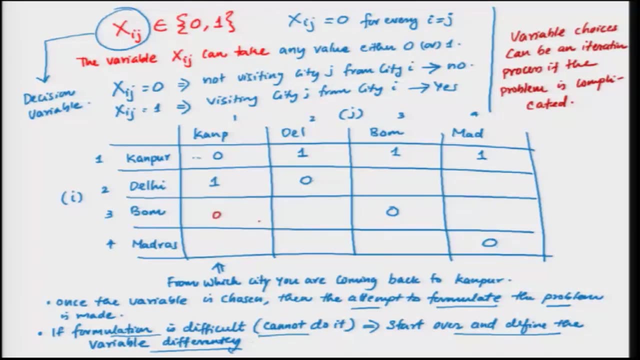 Okay, Okay. So in this case, what we are trying to do is, if you think about this problem, instead of looking into this cost structure, what we are doing is we are actually converting this into a 0- 1 problem. okay, Like this: if you can say all of these are zeros, okay, then you are saying that this is 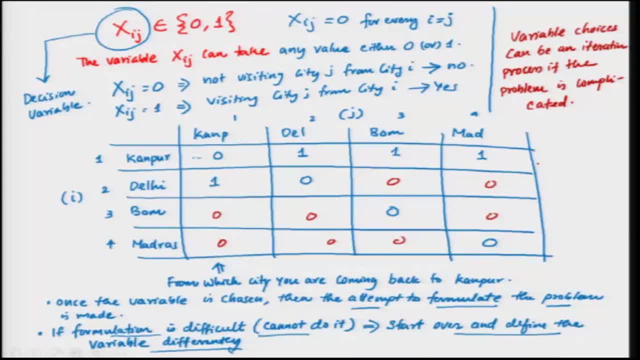 the order in which you are visiting. whether this visit is okay or not, that is a different story. but yes, this actually means that you are travelling from Kanpur to Delhi, Kanpur to Bombay, Kanpur to Madras And returning back to Kanpur. Okay, 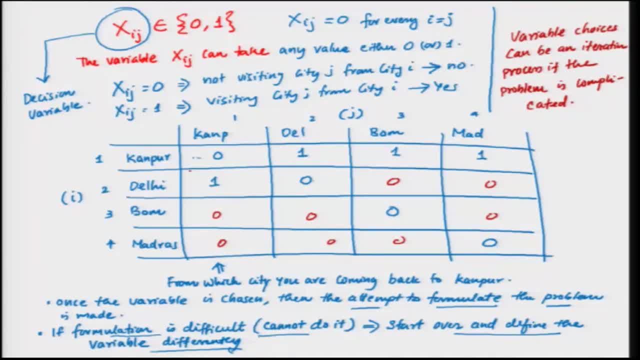 To Kanpur from Delhi, kind of a thing. okay, This might not be a feasible thing, or it might not be something that makes any sense, but for the time being, this is one option, because you have no other thing that prevents you from choosing a tour like this. 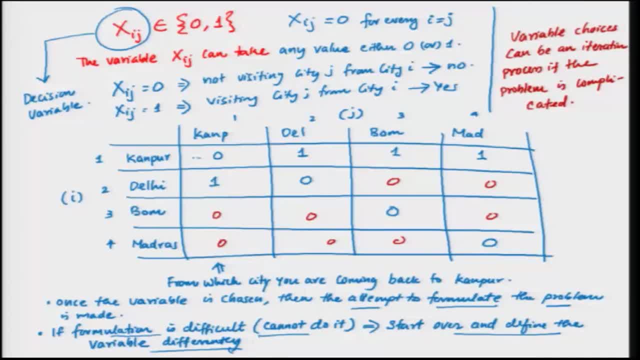 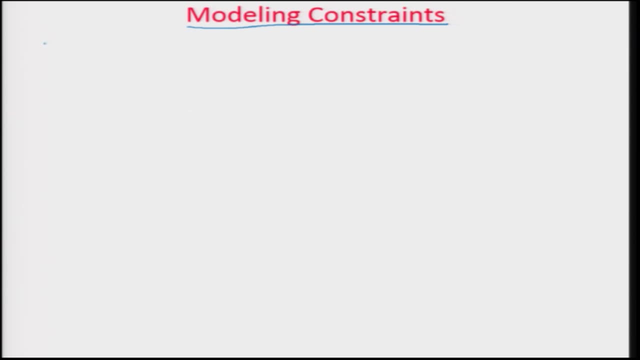 So I can actually make a tour like this, okay, So then, the second part of it is now. the next most important part of this problem is all about the how do you model the constraints, or the modelling of the constraints. Okay, Now we deal with the condition, with the requirement, with the requirement that each city, each city- 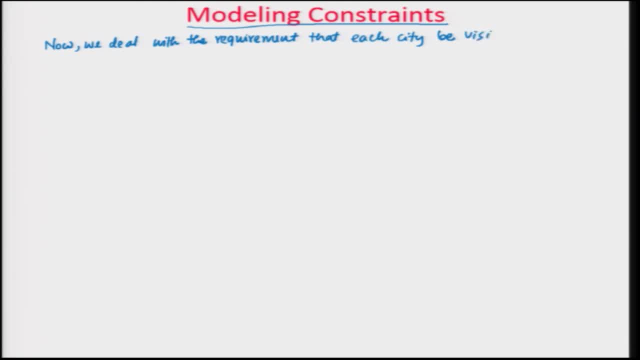 be visited only once? okay, We want to visit each city only once. okay, You do not want to visit only once? Okay, You want to visit more than that. So how would you do that? okay, So let us take a, for example, this case of the city 2, which is Delhi. okay, 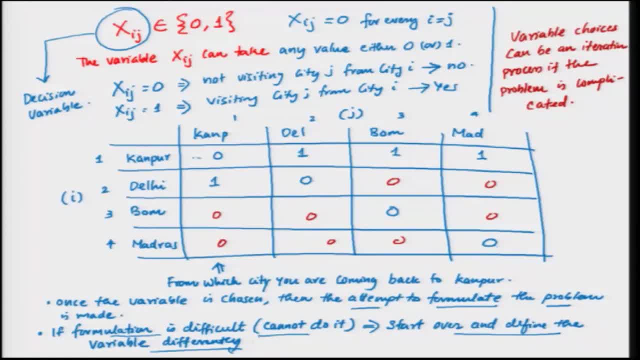 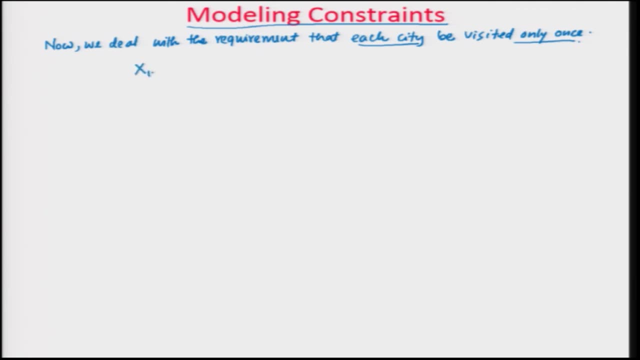 Think about this, then the simplest way to think about it is: if you want to ensure that the city, Delhi is visited only once, there should be only one in this column, right? only one in this column. or another way to say is, if I say this, something like this: X, 1,, 2,. 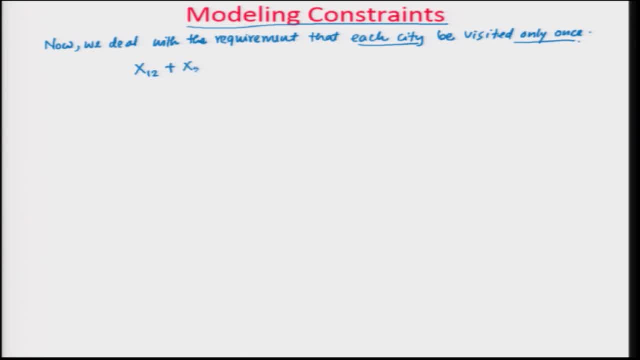 plus X 2, 2 plus X 3, 2 plus X 4, 2 is equal to 1.. If I say this, what am I saying here? this is your 2, the column number 2, okay J. So your J is 2, okay in this case. 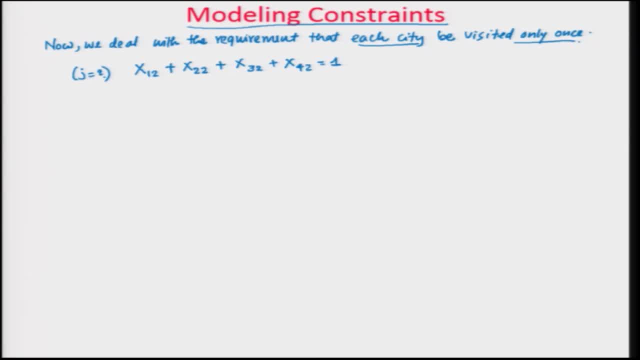 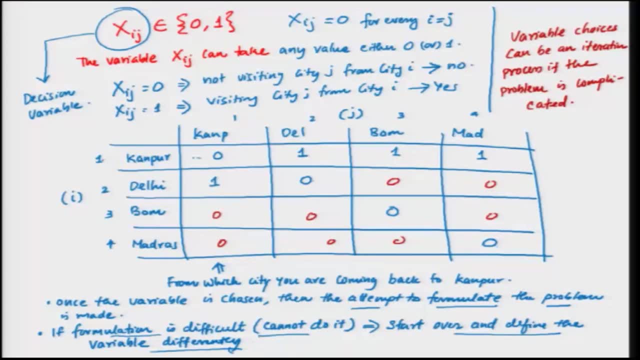 So in this case, you can see that this J is equal to 2. in this case, it remains 2,, 2, 2. the Jth position always remains in 2, okay, And the Ith position varies from 1,, 2,, 3, 4.. 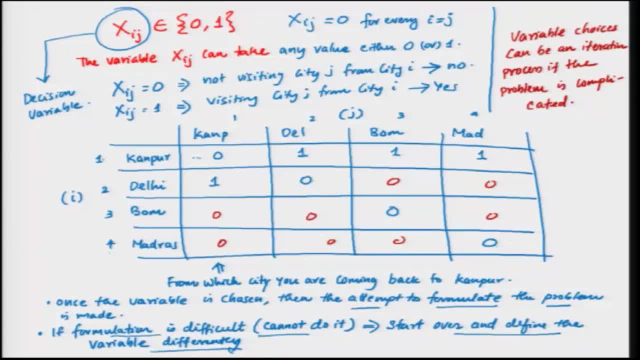 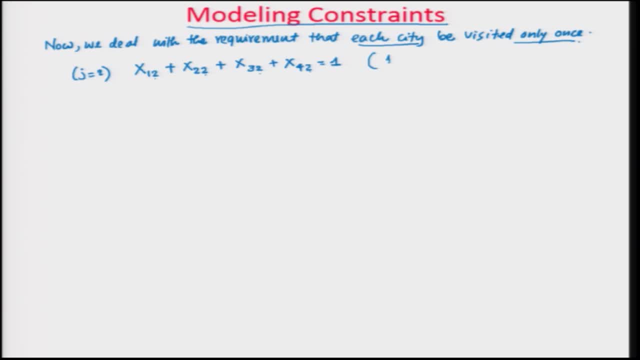 So each one of this, okay: X, 1,, 2, 2,, 2,, 3,, 2,, 4, 2.. If I sum all of them, we are actually summing 1 plus 0 plus 0 plus 0, which should be equal. 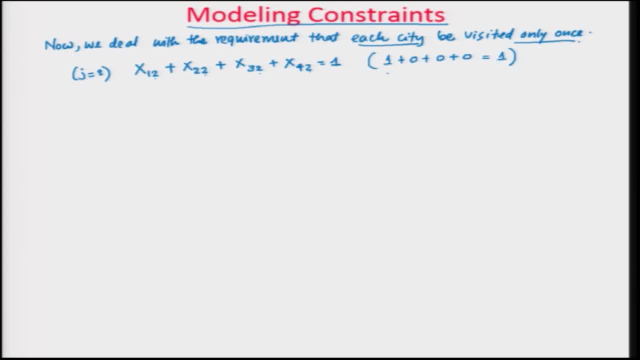 to 1.. If we can create right a mathematical constraint like this, then what we are actually saying is: no matter what, each city is visited only exactly only once, okay, Okay, So what we require, what we need for our model, our model, is a general mathematical expression. 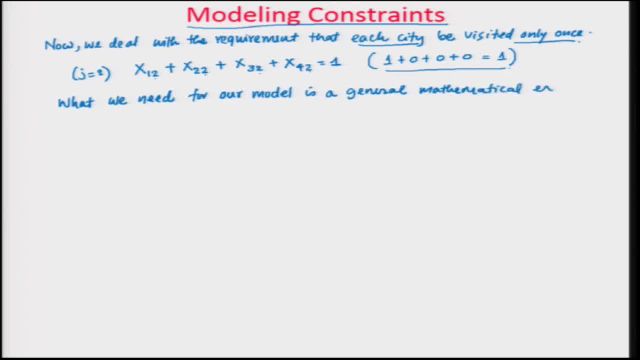 mathematical expression. mathematical expression that encodes: Okay, That encodes, Okay, That encodes, Okay. Okay, That encodes this information, okay. So I can say that for the city of, let us say, for that matter, city of Bombay, which is to 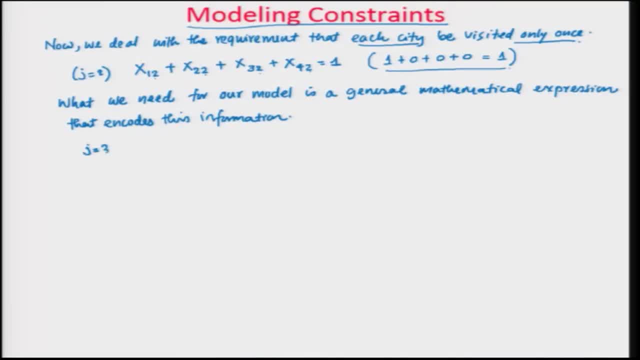 be 3, I can say that when J is equal to 3, I can also say that X 1, 3 plus X 2, 3 plus X 3, 3 plus X 4, 3. okay, this should be equal to 1.. 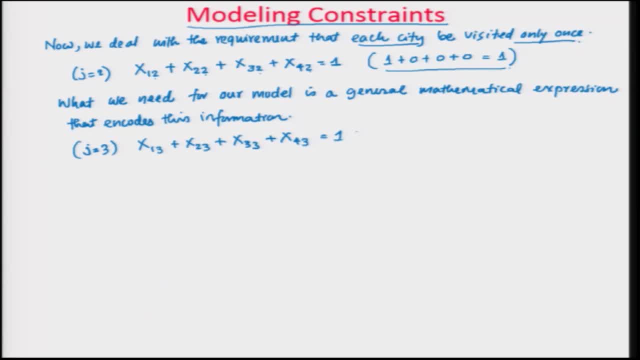 So, since you can approach this, You can apply this same logic to any column. you can write this as this purely mathematical expression: okay, Translated as. translated as: okay. sigma summation of I is equal to 1 to 4, X, I, J, I comma, J, okay. 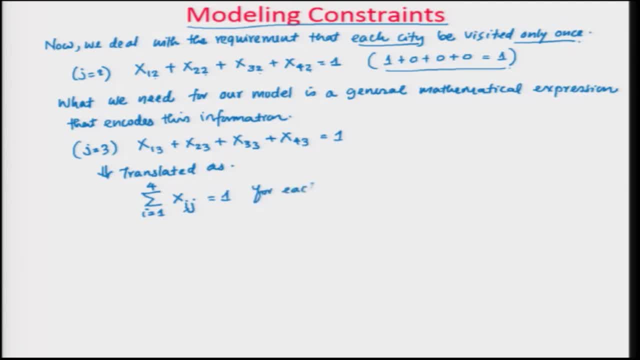 equal to 1. for each fixed J, equal to 1.. Okay, Okay, Okay, Okay. So what? you are saying? that for each fixed J, the value of J remains fixed. from 1,, 2,, 3 and 4, the value of I can change from 1 to 4 for each value of them. the summation, the: 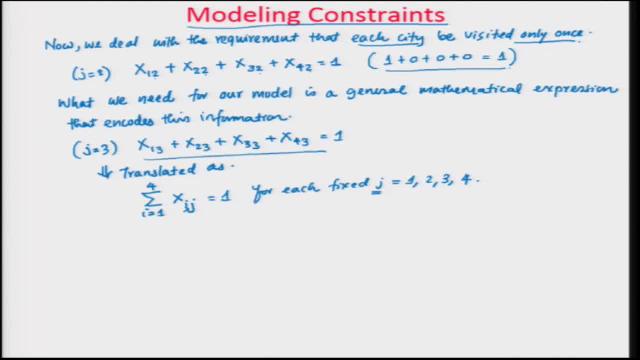 sum of them should always be equal to 1. okay, Or what it says is: there is exactly 1, so in a, in another word, you are saying is that: okay, there is exactly 1.. exactly 1 cell in the column of the city that has a non-zero value. non-zero value in this. 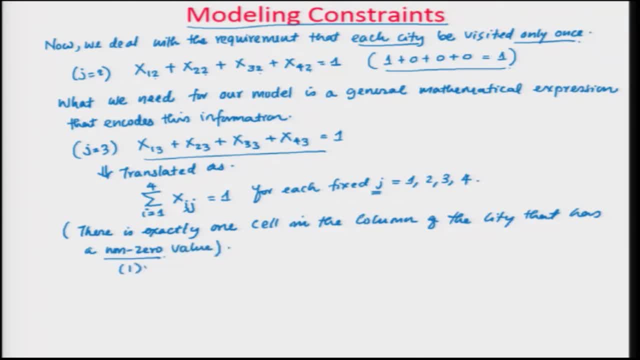 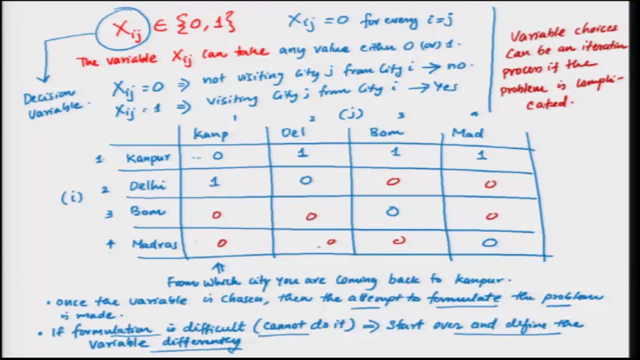 case is 1, okay. non-zero value is 1 in this case, okay. I hope you guys understand what I am talking about. so, each column- if you do this, so we think about it, yes, in this case it is. this whole column- sums to 1, this sums to 1, this also sums to 1, this also. 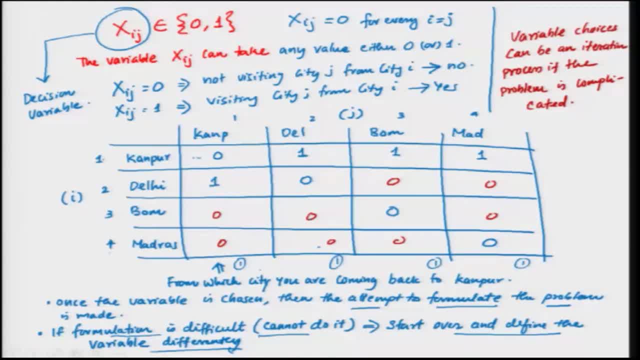 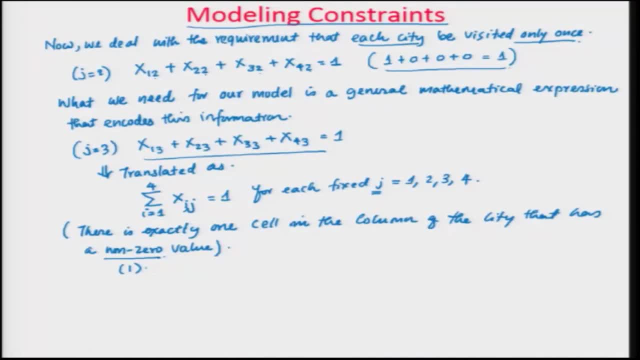 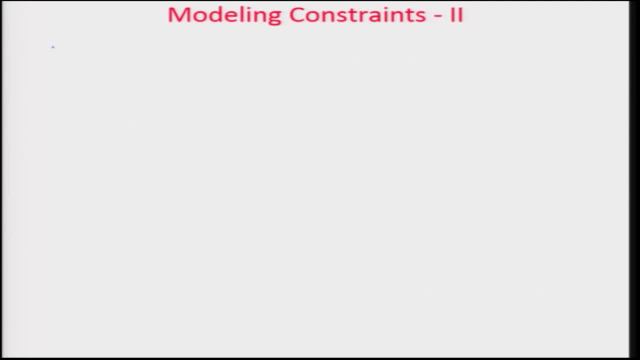 sums to 1, this also sums to 1.. So, ideally speaking, this solution says that, yes, you are visiting only each city once. okay, fine, so this is the first part of the approach. okay, So in our case, the earlier constraint constraint took care of the, took care of the of the. 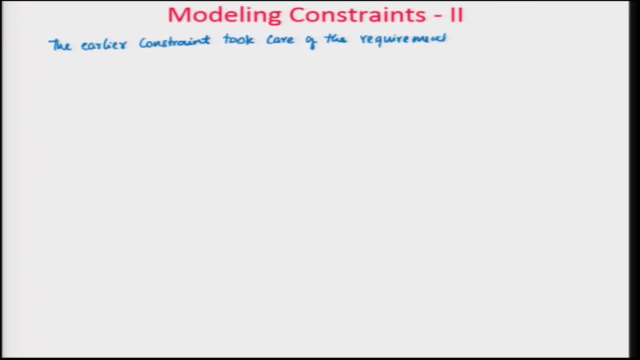 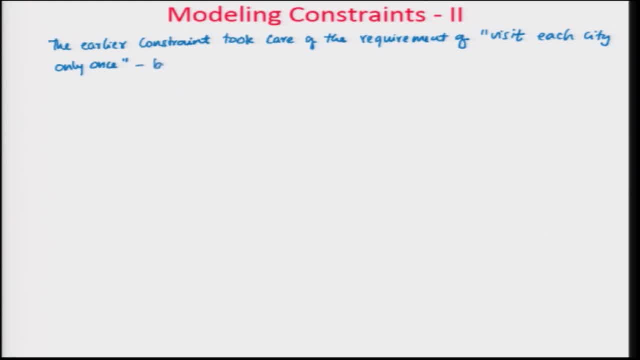 once okay, but fails to ensure that the resulting trip is a round trip. So, for example, what I can say here is the previous example that we draw. I am just going to draw that small in a small fashion right here, not a large one, we will draw a small. 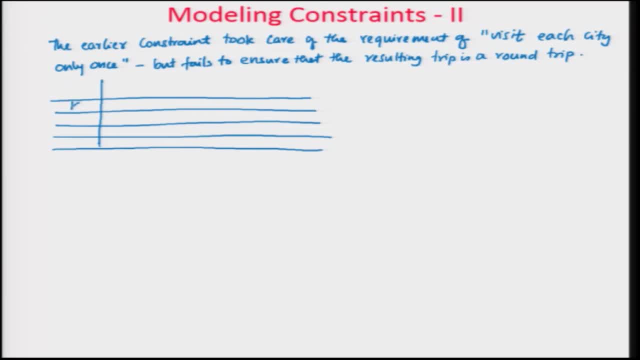 matrix. okay. So this is your: Kanpur, Delhi, Bombay and Madras- and we have already started abbreviating and I am lazy in this regard. so that is what we are doing: Kanpur, Delhi, Bombay and Madras. So what I did earlier was this: okay, everything else was zeros, okay. 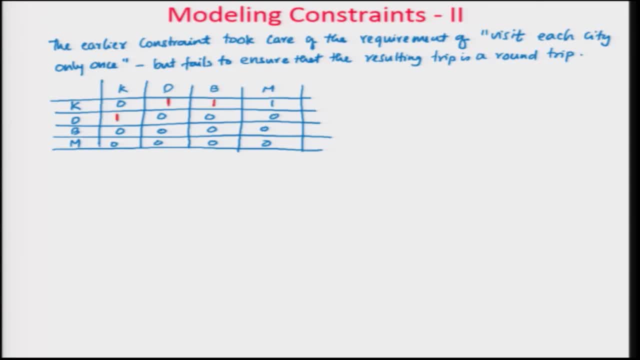 In this case, the ones are here: 1,, 1, 1. okay, we have 4 ones in this regard and the rest of them are zeros. okay, So, while this ensures that each city is visited once, The option that you are having here is Kanpur Delhi. okay, then you have is Kanpur Bombay. 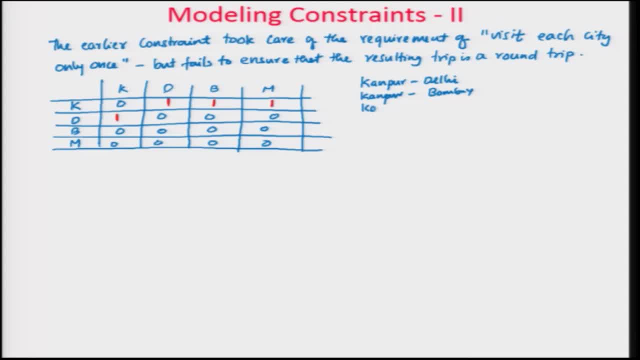 okay, and then you have is Kanpur, Madras, and then Delhi, Kanpur. So by this option, there is no way you can ensure a round trip. You are never doing a round trip because you want to visit only the city once. Yes, you have visited city once, but the point is that this does not result in a round trip. 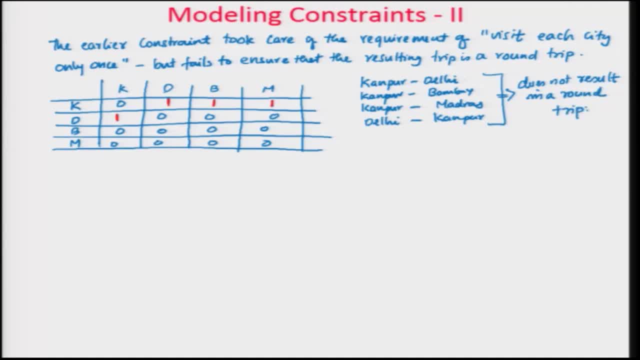 okay, Even though you can visit the city, each city, exactly once, but it does not guarantee a round trip, okay. So what are we saying? is that? so what? in words? if you translate this, This means This: This, This Assignment or this choice: okay, represents it, represents this choice, represents the. 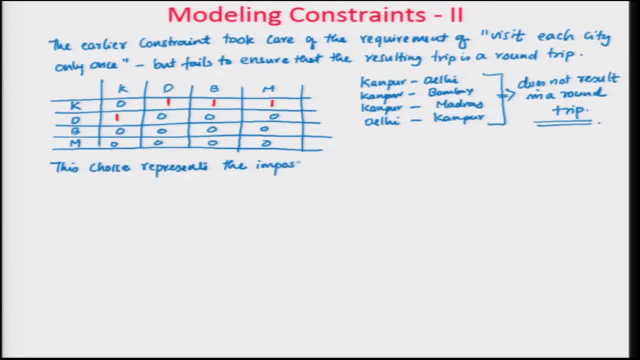 impossible scheme. The impossible scheme of visits. Since Kanpur is The. The is the origin for all 3 cities, but the destination is only from Delhi. okay, So you can see that in words in English: your origin of each 3 cities visit is from Kanpur. 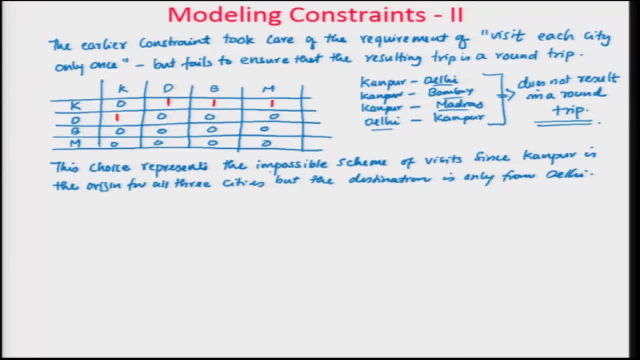 but the destination back to Kanpur is only from Delhi. So this gives you results into what we call as an impossible scheme. okay, or this is also what we call as an infeasible solution in the optimisation terms. When somebody says an infeasible solution, what we are talking about is an impossible. 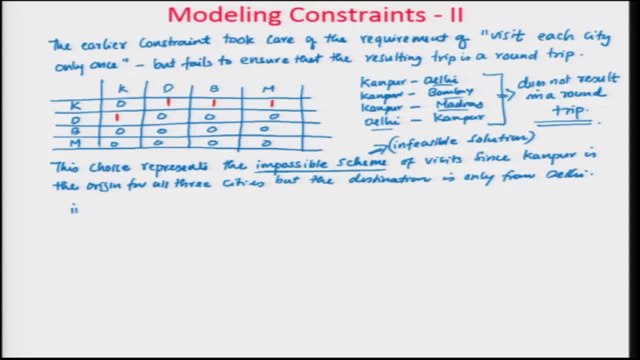 scheme or a set of values. So an infeasible solution implies, okay, a set of values for the variable. that results in an impossible scheme. okay, So, the impossible scheme is also known as infeasible solution in this regard. okay, So what? the solution that we draw here is an infeasible solution or an impossible solution. 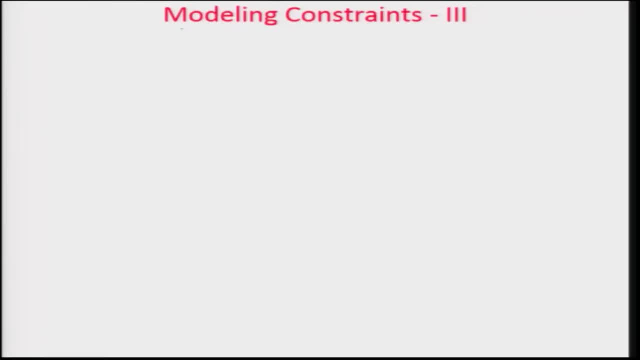 in that regard. okay, So how can you address this? So, to address this, to ensure that infeasible solutions are not happen, we also need another constraint. We also require another constraint that ensures that, ensures what does this constraint should ensure that the constraint should ensure that each city, each city serves as the origin for 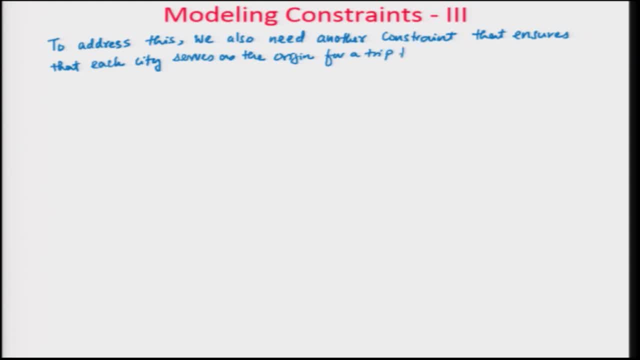 a trip. Okay, So let's choose one city. this means you can't have two cities or multiple cities- one another city, So you cannot have one city. So this implies told having the same city as origin multiple times. So what are we doing? 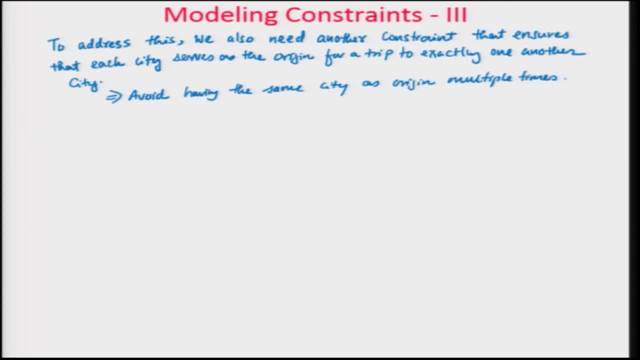 Now let's see one more example. So you are basically saying that: exactly one. so your city serves any city. each city serves as the origin for a trip. exactly once, certainly one to another city. okay, So if you want to do that, then the way to do it is, if you draw that diagram that we 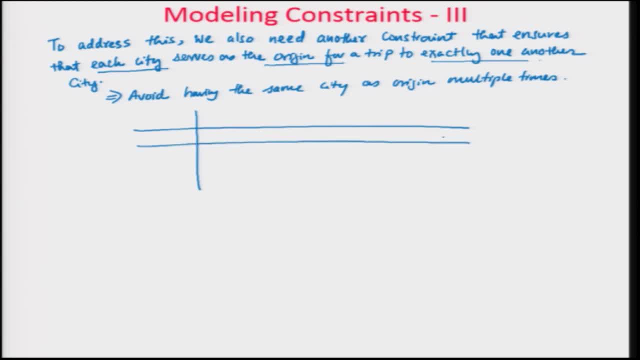 drew earlier, okay, which is something like this. I will try to draw nicely today. So this is your from and to. okay. from to: this is Kanpur Delhi, Bombay Madras, I believe. and Kanpur Delhi, Bombay Madras, okay. 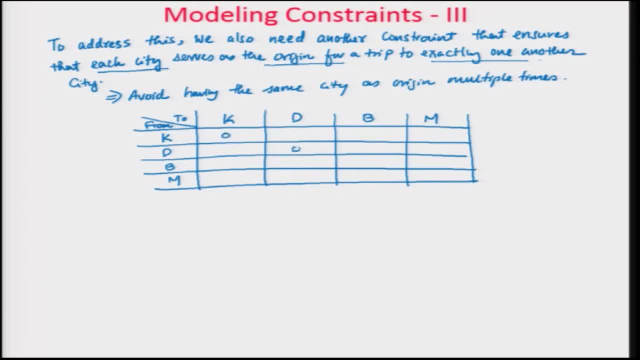 And the. what we were saying is that all these diagonal elements are 0 because the tour within the city is not allowed. and then let me put all these 0s in red colour- actually not 0s, the ones in the red colour. So this was the scheme that we came up with, and then the rest of it was all 0s. okay. 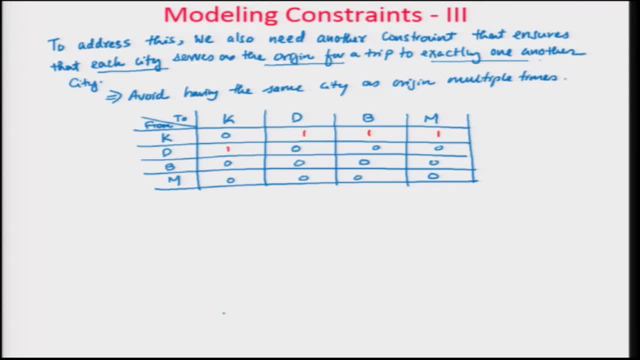 This was the impossible scheme. where you are, this results in a violation of this scheme credit. so these 4 pieces of x dot what we are established, each and every piece, as to stepped 500 square feet. And then what we came up with is this: by this condition, origin for each of trip is exactly. 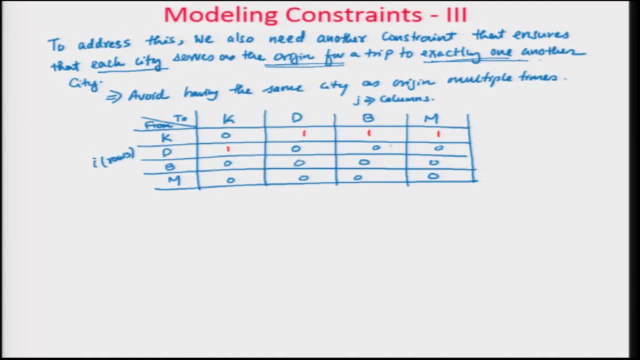 one another. So what we have done is: this is your j, which is the columns, okay, and this is your I, which is the rows. So we have ensured the sum of the columns should be individually one. so this should be sum to 1,. this should sum to 1,. this should sum to 1,. this should sum to 1.. 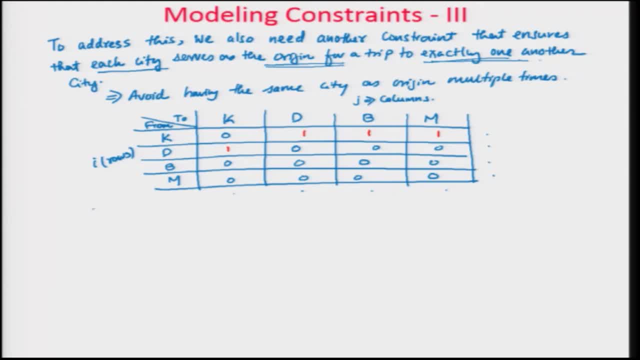 Now you have to ensure that this is 1.. You have also to ensure that the rows are also summed to one. write that So I can say it, as if I have to sum this row, then I have to say it as: x11 plus x12 plus x13 plus x14 is equal to 1.. So 11 is this column, this is 11,, this is. 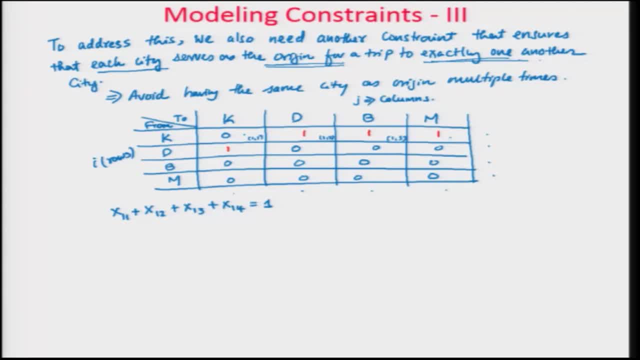 1, 2,. this is 1,, 3, this is 1, 4.. It should sum to a maximum value of 1.. In this case, if you think about it, it actually sums to 3, which is a violation of this. okay, So then? 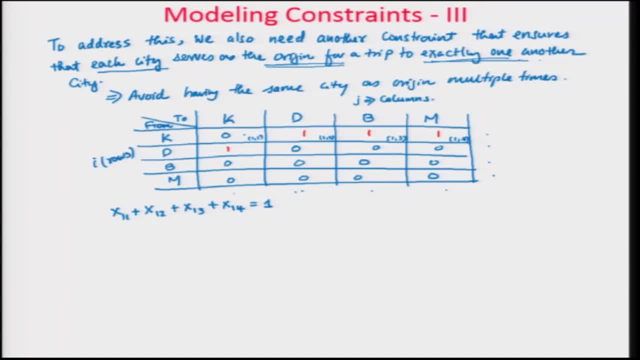 what will happen in our case is we will have to change this. So one way to do it is: I am just going to change this portion only so that you have an idea. okay, I am going to change these to zeros and zeros, And then what I am going to do is: I am going to change this portion only So that you have. 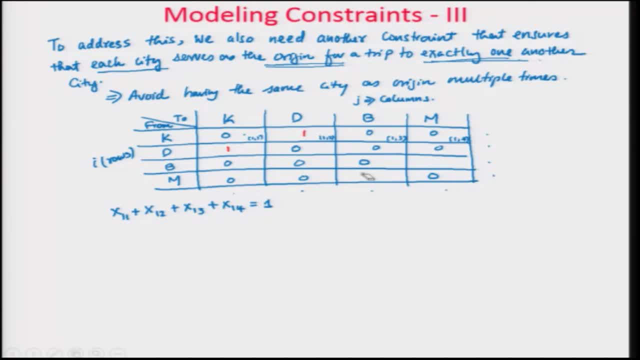 an idea. okay, I am going to change these to zeros and zeros, And then what I am going to do is I am going to just change these to red colour 1 and 1, okay, So now, if you think about it, I have a scenario where each column has once summed this fashion: okay, 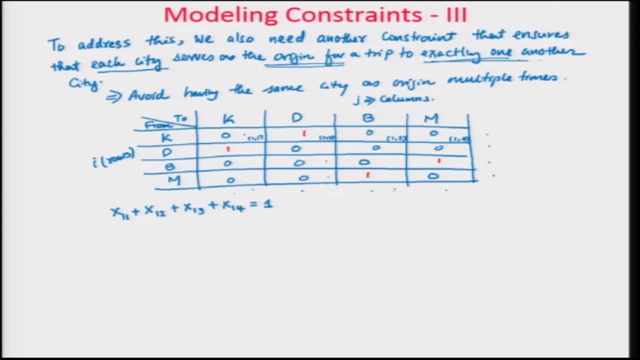 You have a one summed this fashion. you have one summed this fashion. one summed this fashion. one summed this fashion. Same way, you have a one summed in the row fashion as well. okay, So if I write this constraint, then I can say it as x11 plus x12 plus x13 plus x13 plus. 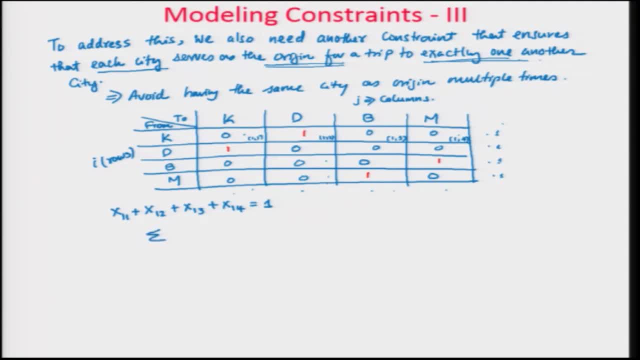 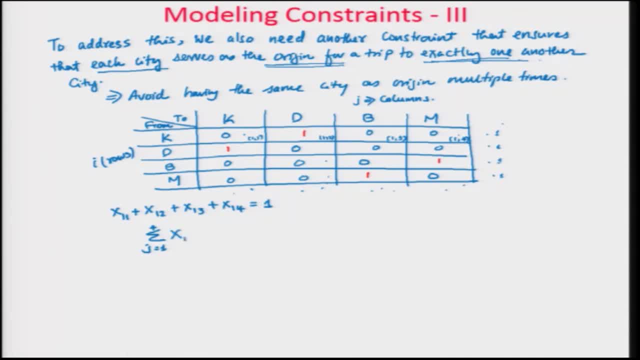 But the row will remain the same of xij i, comma j is equal to 1. okay, For each fixed i equal to 1, 2, 3, 4. okay, So you are basically mathematically saying that this is the same. each row should also sum to 1, so that, exactly, you will have something called as a each city. 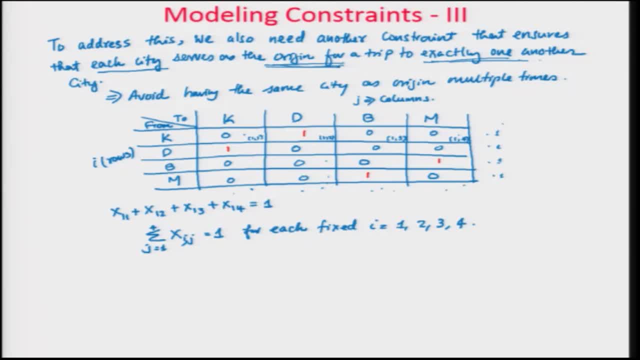 should serve as an origin for a trip of exactly one another city. okay. So if you think about this, then the trip actually is something like this. at this point you can see it as you know. it is a. you can say: it is Kanpur to Delhi. okay, and Delhi to Kanpur. 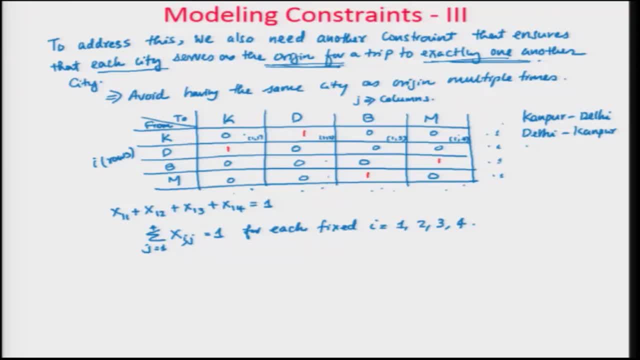 okay, then you have Bombay to Madras and Madras to Bombay. okay, yeah. So, if you think about it, Yes, you have visited each city only exactly once. okay, but then you did not visit them in a complete tour. you are not completed. so, from Kanpur to Delhi you went, and from Delhi 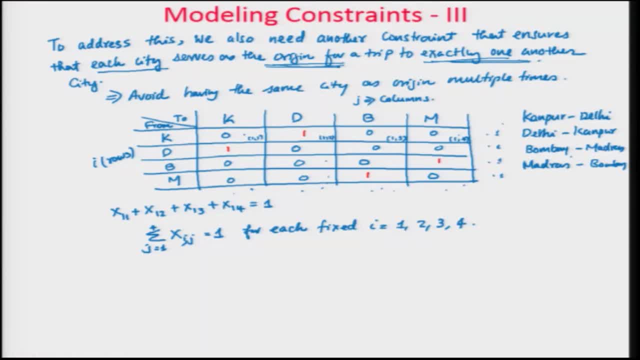 to Kanpur. you came back, then somehow you reached Bombay, and then from Bombay to Madras and Madras to Bombay. so you violated. so this is not equivalent to the tour that we told earlier. so this is this has actually two. there is one cycle here and then there is another cycle. 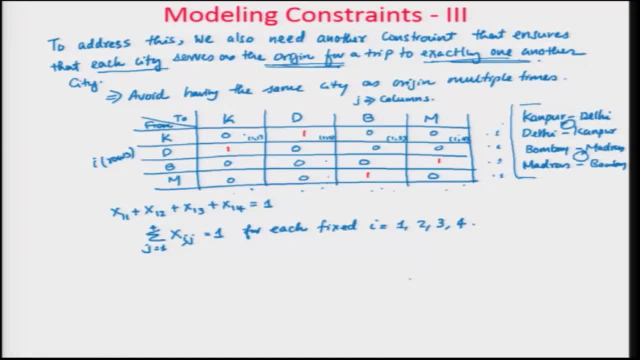 here. okay. So what we have here is: Yes, we got a round trip, we got a round trip, but not a true round trip due to the many round trips inside, mini round trips. okay in the solution. So what you are saying here is that because of this mini round trips, you are not been. 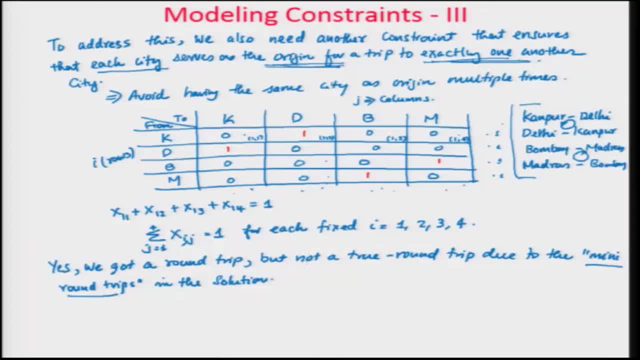 able to, you are not been able to reach a true round trip. such kind of behavior, these kind of things are called as okay cycles in the graph, okay. So when you have these kind of cycles, where your solution- yes, it will satisfy these constraints, the currents constraints of ensuring that these cities only visited exactly once, but 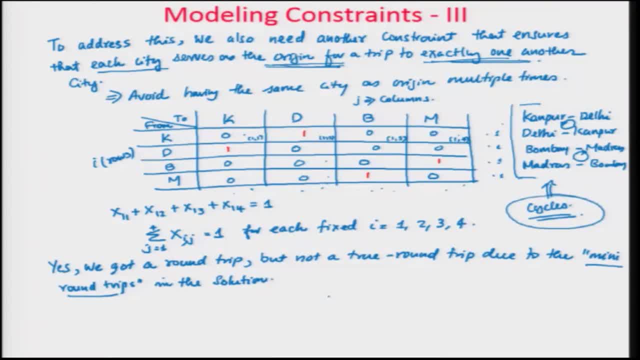 you might not get a true round trip yet. okay, So to ensure that you have, you can get a true round trip, you need to, you know, enforce a constraint, okay. So now one other way to think about it is: how do you enforce this constraint? enforcing 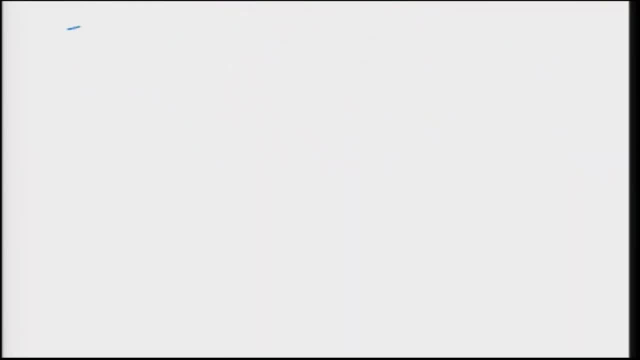 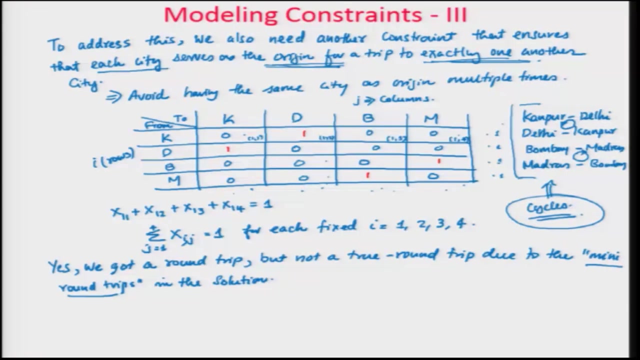 the constraint is The true round trip. the true round trip can be enforced with the constraint, enforced with the constraint, with the constraint. So like, for example, if you think about here it is: this is 1, 2, 3 and 4, this is 1, 2,. 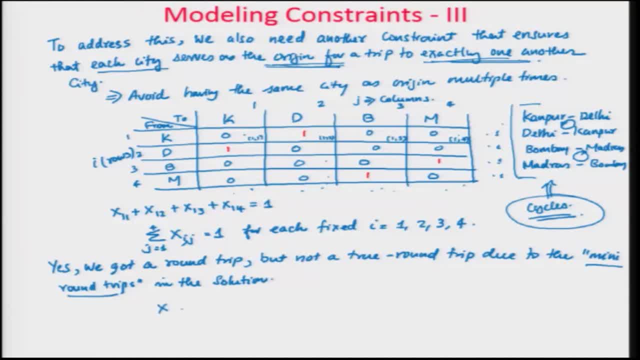 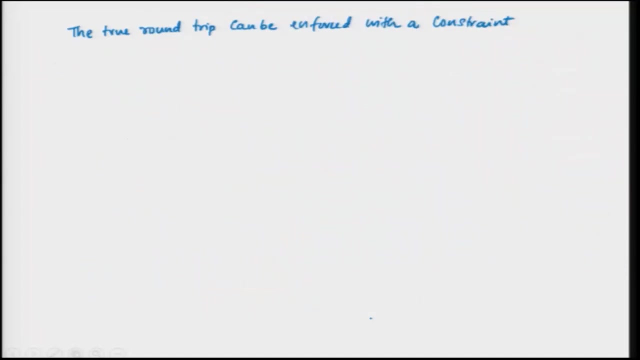 3 and 4.. So the values you have here is x12 equals x21 equals 1. the other one is: x34 equals x43 is equal to 1.. So these are the two ones that we have. okay, So what we are trying to do is, if you try to create a constraint saying that, so this 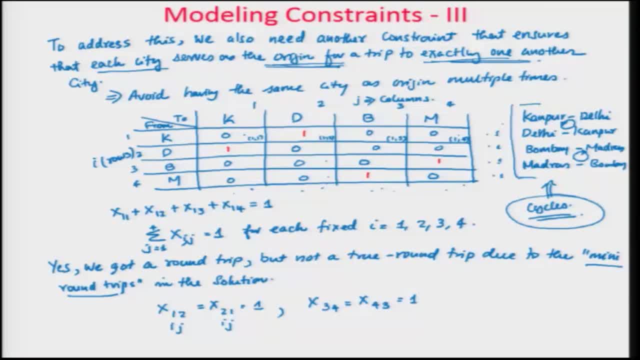 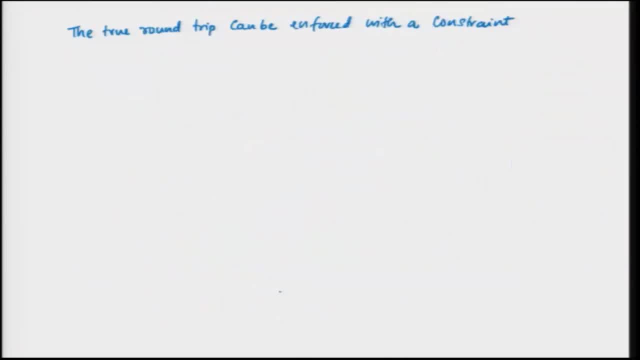 is your i and j. So you think about it: the ij and ji. if you interchange these guys, okay, then you are getting the same stuff. So if I say that xij plus xji, okay. If I say that it is equal to 1, that means I am really, instead of let us not talk about. 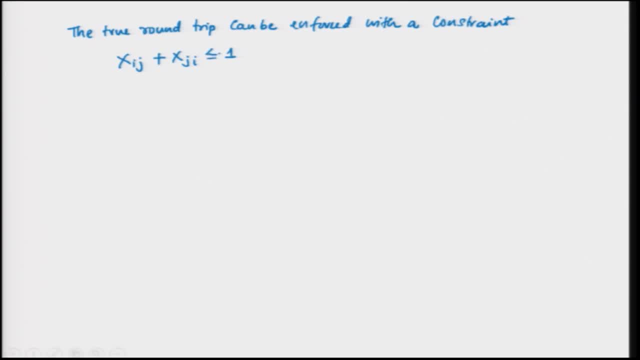 equal to 1. if I say it is less than, or equal to 1. if I say this, that means the maximum value I can take, this This is 1.. So, if any case, if this case is 1, then that means this should be 0.. 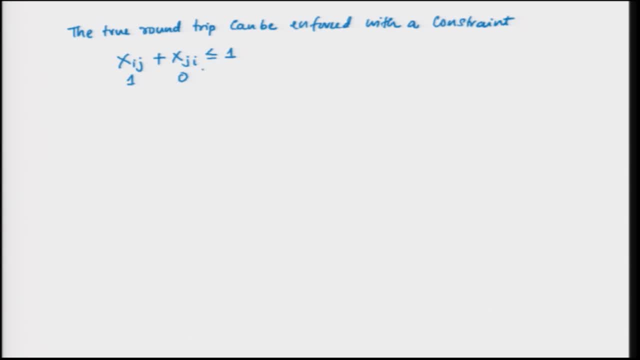 So that will ensure that the cycle will come not happen. okay, So this is for all. i equal to 1,, 2,, 3, 4 and j equal to 1,, 2,, 3, 4.. So all possible options. 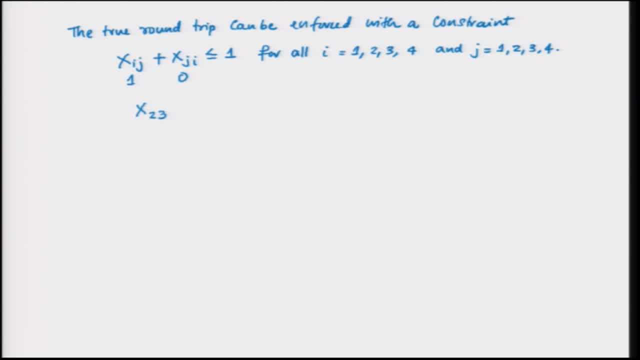 If you say x234.. If you say x23 is equal to 1, then x32 should be 0. that is what we are actually saying. This prevents the occurrence of occurrence of mini cycles in the solution. okay, So as we drew earlier, 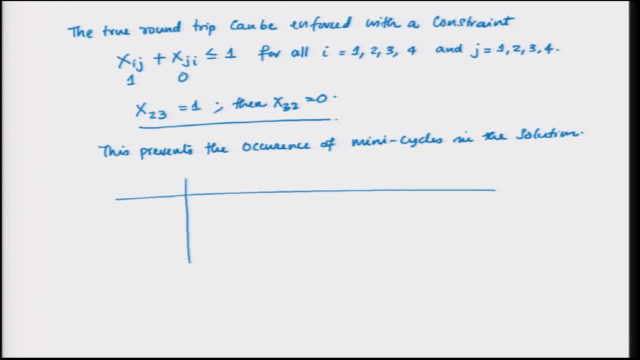 The graph or the table. okay, we will draw once again here. This is your: Kanpur, Delhi, Bombay, Madras. Here is your Kannpur, Delhi, Bombay and Madras. okay, and the solution that we had at this point was this: 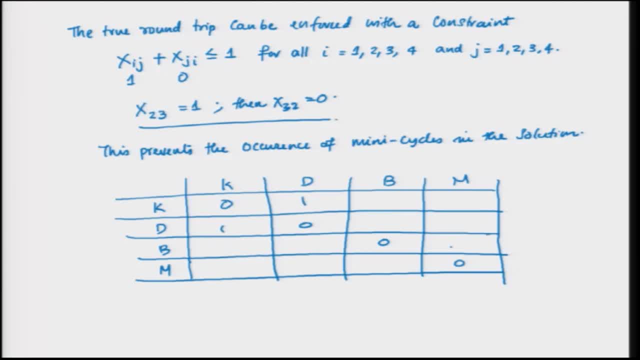 Okay, and we had, it was this right? and everything else was zeros, okay. So let me do this one so that you- and it makes life easy to understand- 1 and 1,, 1 and 1, okay. So when you enforce this constraint, when you put this constraint into picture, then when 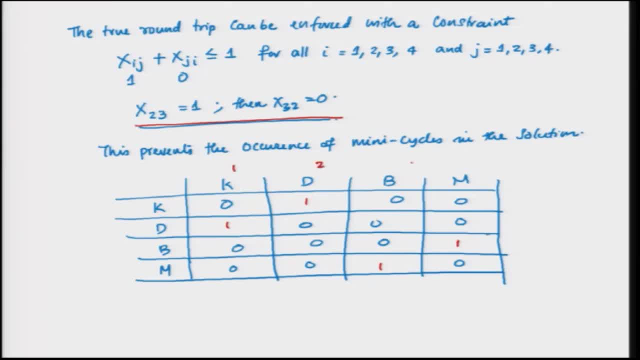 you say: this is 1,, 2,, 3 and 4,, this is 1,, 2,, 3 and 4,. this is your i and this is your j, okay. So when you say x, when you have, this is 1, 2, okay. 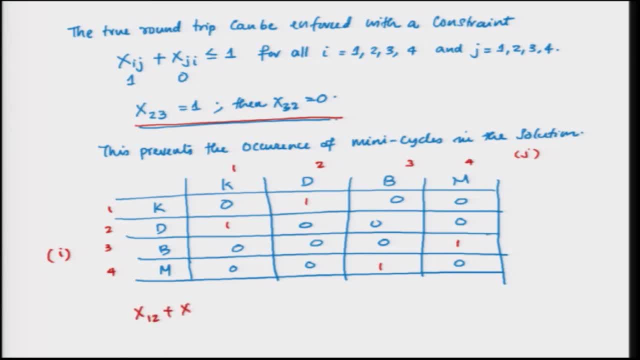 So when you say x 1, 2 plus x 2, 1 is less than or equal to 1. if I say this, when you look into this, x 1, 2 and x 2, 1 should be less than or equal to 1 means one of this. 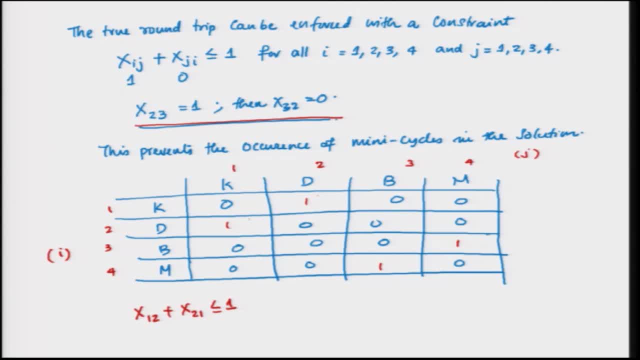 has to be 0. So I had can. I can say: either I choose this, then this should become a 0. okay, if that happens, then what I will have to do is I will have to make something else as a 0. So I might have to maybe do this. if I do that, then I will say: okay, fine, then I this will. 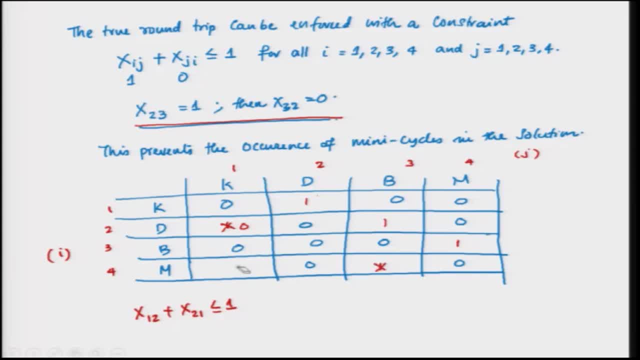 violate the other constraint. So I might end up making this and moving this to what we call as a 1. in that process, I will probably get a 2 out of this. So if you think about this assignment, then what would happen is it is from contour to. 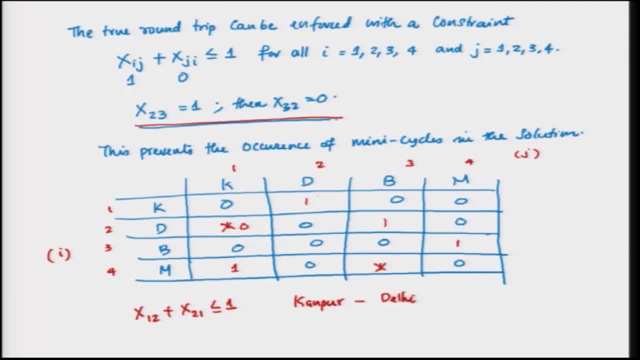 Kanpur, Kanpur to Delhi, and from Delhi we are going to Bombay, and from Bombay we are going to Madras and from Madras we are coming back to Kanpur. okay, So this actually gives you a true tour, where you are visiting each city only once, okay. 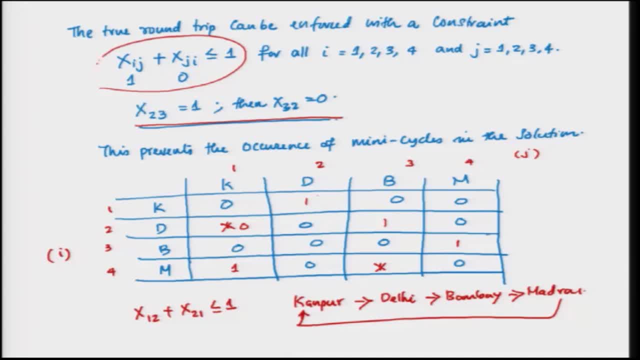 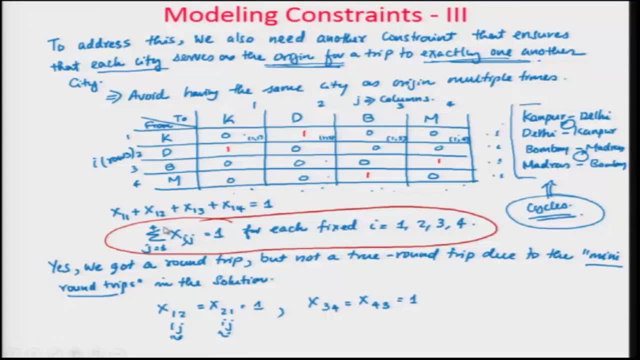 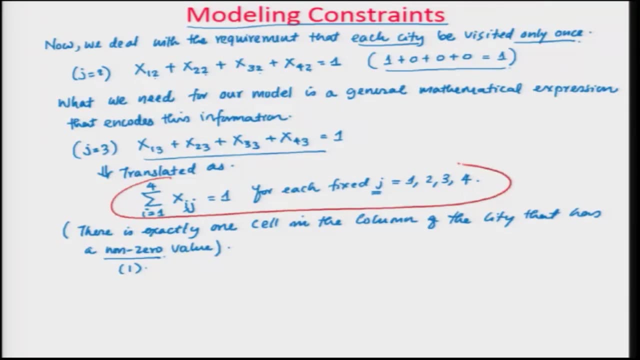 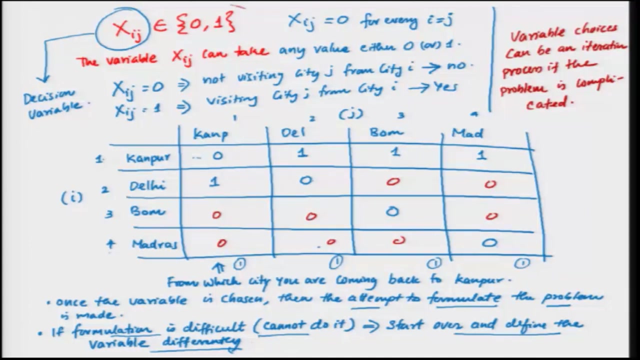 So all these things put together, okay. So this is your one constraint. Then in the previous slide, we had a another constraint: right here, right, this is another constraint. then, if you think about the previous one, we had a constraint which is right here, okay. Then in the previous slide, we also had a constraint which is this: okay, they are both. 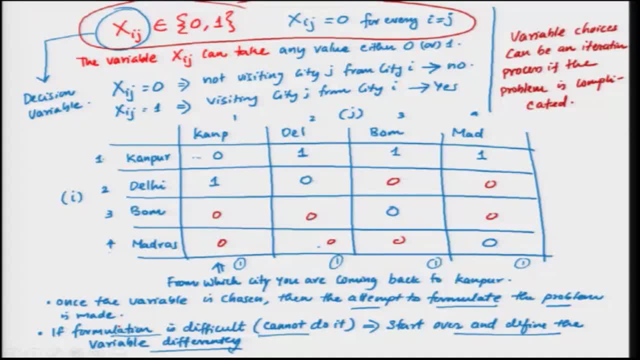 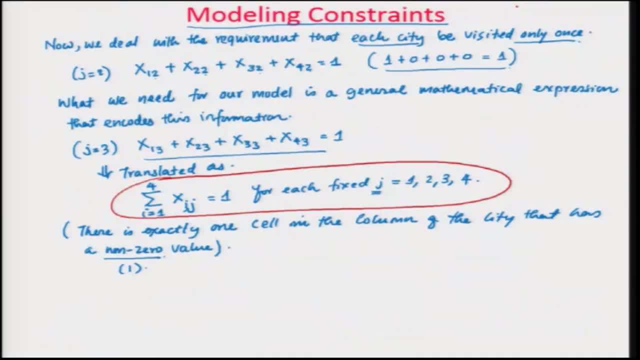 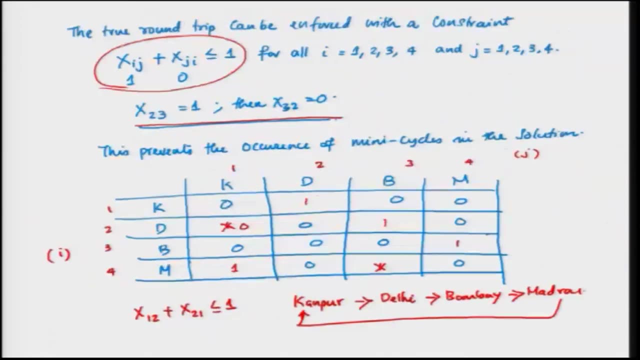 elements of 0, 1 and the other one is not equal to 0. okay, So these constraints put together, If I call this as constraint 1, okay, and this is constraint 2: okay, and this is constraint 3: okay, and this is constraint 4: okay. 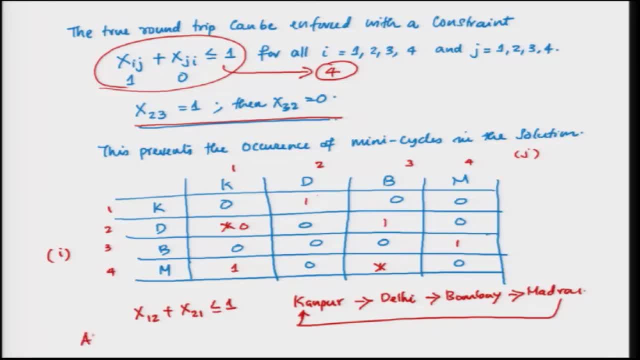 Then with these 4 constraints, put together all the 4 constraints together results in a round trip with each city visited only once. Okay, Fine, So there is one homework question for you guys. okay, So this is a homework question you have to think about. it is homework, okay. 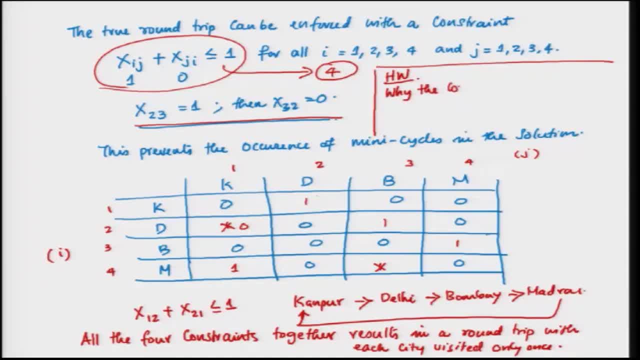 Why the constraint 4: okay, should not be written as. should not be written, as Xij is equal to Xij plus Xji is equal to 1. okay, Why writing this is not the right thing to do? okay, So think over it and try to answer this question. 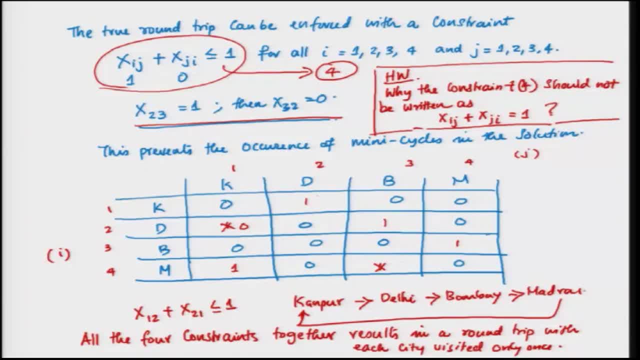 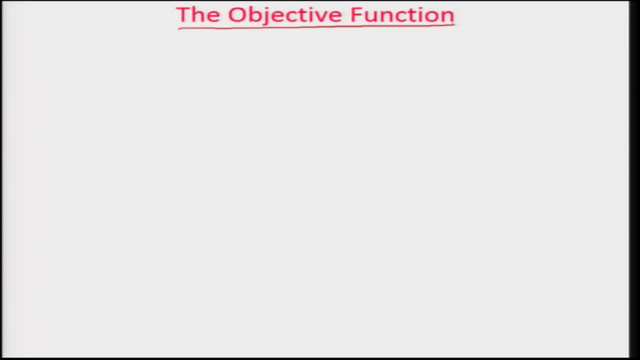 This is your homework question. okay, alright With that. now, okay, we get into the last part, which is called as the objective function. okay, So the objective function. so we are gone through now the variables, We have gone through the objective function, We have gone through the constraints and now we are at the objective function. okay, 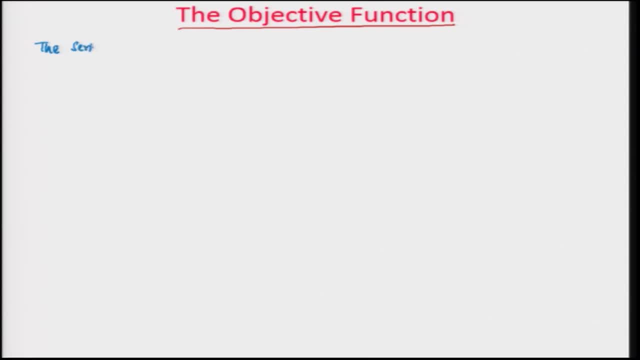 So the series of constraints, of constraints, the series of constraints defined earlier. So the constraints that we defined earlier allowed Okay, Okay, Anybody else okay. So the constraints of constraints are not the same rules, The constraints of constraints in how lots of things happen, kind of constant澤. 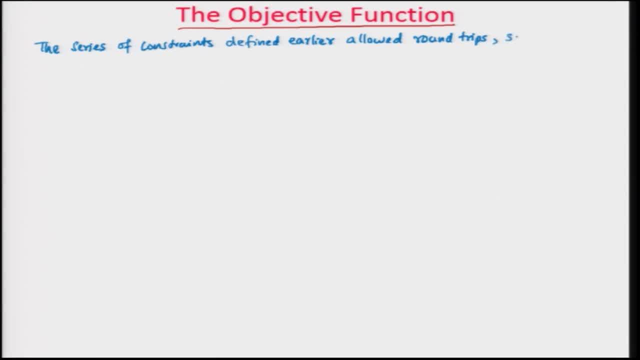 Why I am some kind of weird. I am believing they are not risks. What I am trying to say is why I am telling you this question: know functions, museums before operations are things, but don't Черin film in the past what or what you are. 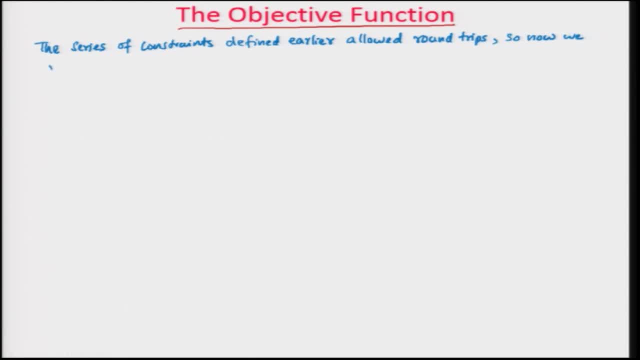 going to do with things after changes or what is going on is going to be difficult to say right is not working out Why I am so sorry. I am sorry, Chetra. So the first thing that I am trying to say is why we have similarly defined a 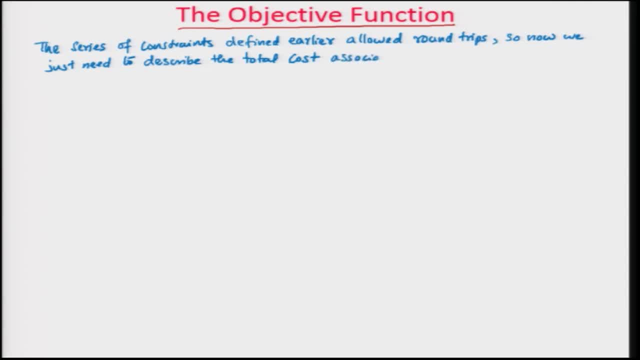 certain. this is called as a modeled structure. when you have this, you have to conscience what happens where, what you never use it. So if I were to say this was a typical condition, that has happened there, yes, you can see with each round trip. okay, So what we are now doing is: now the constraints allowed us. 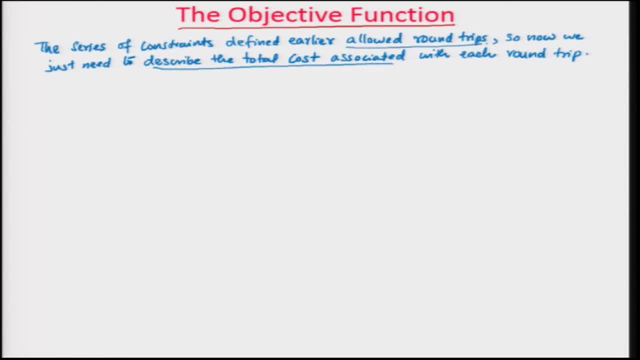 to model the round trip. Now, all we need to do is describe the total cost associated with each round trip. okay, Since our constraints are in terms of Xij, that can take either 0 or 1. okay, Okay, Now we should describe the total cost in such terms: okay, So how will you do that? okay, 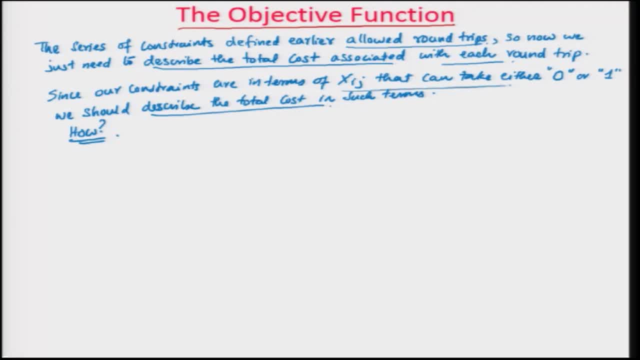 That is the big question. You want to describe the total cost in the terms of Xij, which can take only values of 0 and 1.. Okay, So how can you do that? okay, The answer to this is: we can simply multiply. we can simply. 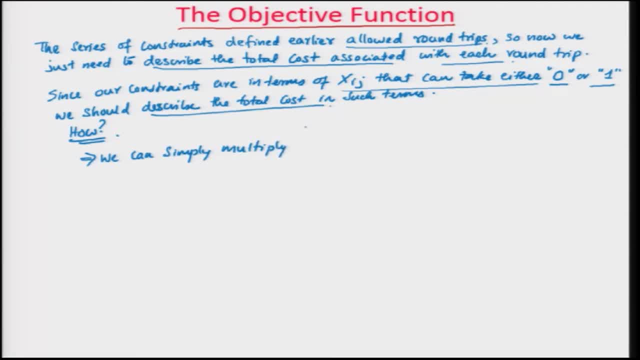 multiply each variable, each Xij, by the corresponding, corresponding cost. Let me call it as Cij, okay, Corresponding cost Cij, and then add it up, okay. So what we are saying here is, in a way, if you think about it, you had your. I am drawing it in together so that you have an. 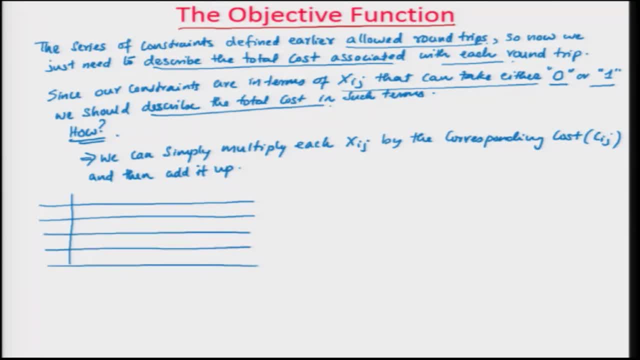 idea of what we are talking about. okay, We had this initial thing okay, where we had Kanpur, Delhi, Bombay, Madras, Kanpur, Delhi, Bombay and Madras- okay, And we had the values in this regard as kept as the cost numbers. we gave it as these were 0000s and we had 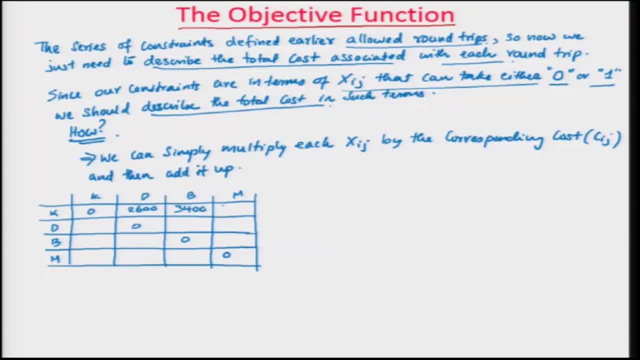 2600, 3400, then 7800.. We had 1800, 5200.. Okay, And 5100, okay, And this was 2600, 3400, then 7800, 1800, 5200 and 5100, okay, And this. 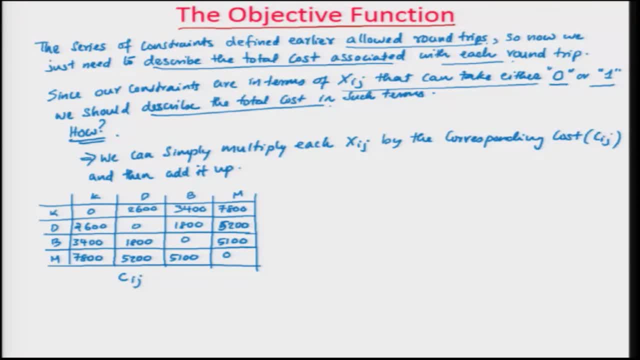 was our cost matrix. So this was your Cij C i, comma j, and you had another matrix. okay, My bad, Let me draw this properly: Okay, 1, 2,, 3, 4. okay, This much Say: 1,, 2,, 3 and 4. okay, So this is the same. Kanpur Delhi. 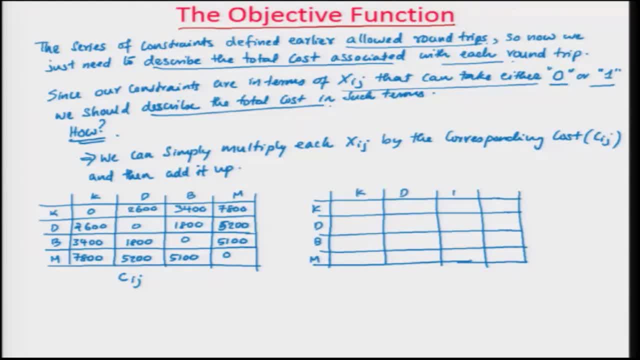 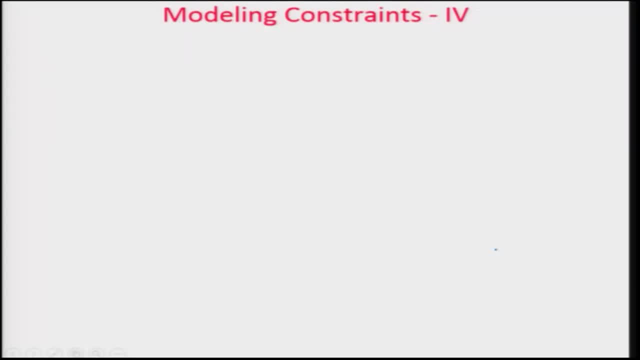 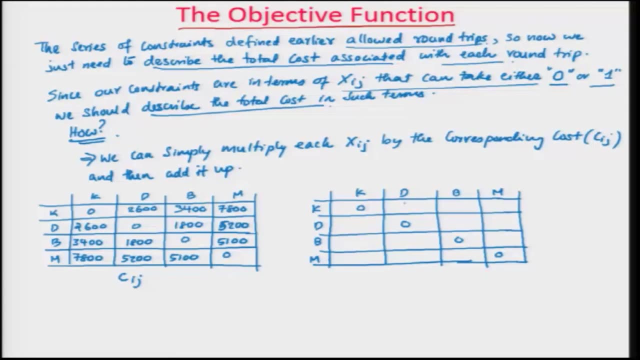 Bombay and Madras, Kanpur, Delhi, Bombay and Madras, And what we had was a bunch of zeros and ones, okay, Okay. So the previous one: we had a 0 and 1.. Okay, 1,, 1, 1 and 1.. So we had a 1 here, 0, 0.. We had a 1 here, 0, 1 here, okay, And 1 here. 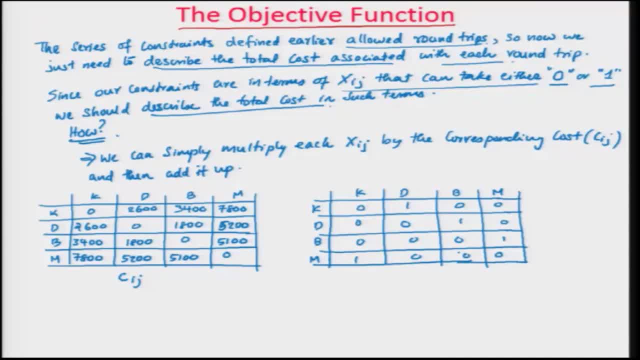 So this was the solution we had. okay, So this is our Xij, My bad, Okay. So what we are actually saying is take the Xij individual values of Xij and multiply it. Okay, And multiply the values of this. So you would actually think about it, as you would think. 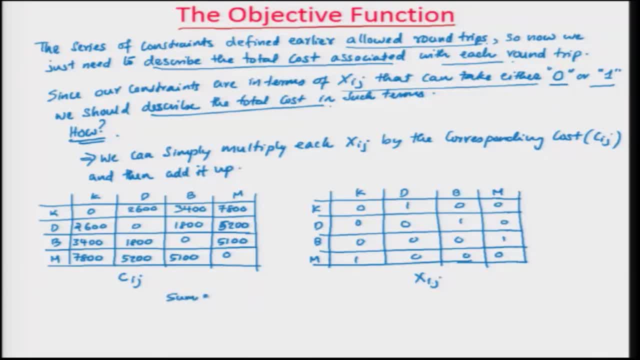 about it as sum all C11 times X11 plus C12 times X12, plus all the way like this to C, this will be 44 times X44. okay, If you think all the, if you sum all these values and put it out, that will be the total cost of the round trip. okay, So you write this mathematically. 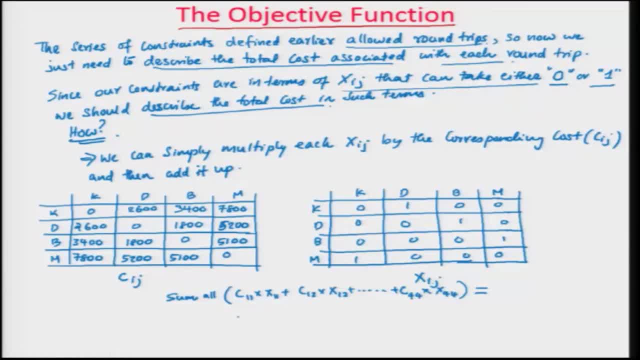 this whole thing. if you want to write it mathematically, I can write it as Cij multiplied by Xij, okay, And what you need to do is you need to sum it 2 times. sigma j is equal to 1 to 4, and. 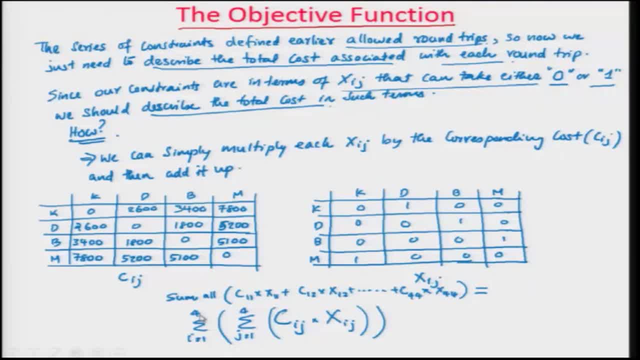 same thing is sigma. i is equal to 1 to 4.. So, for all values of i varying from, i is here, which is 1,, 2,, 3 and 4, and j is here, which is 1,, 2,, 3 and 4.. 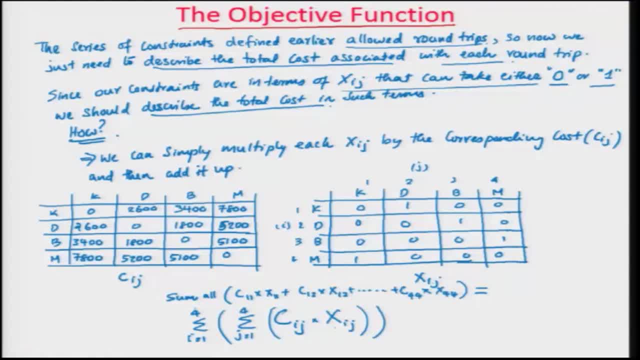 So all the values of i, j varying from 1 to 4 and i varying from 1 to 4, multiply the cost Cij with the Xij, which are 0s and 1s, and sum them up. that will give you the total cost.